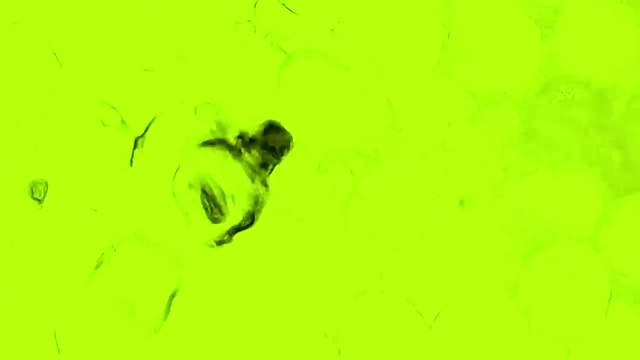 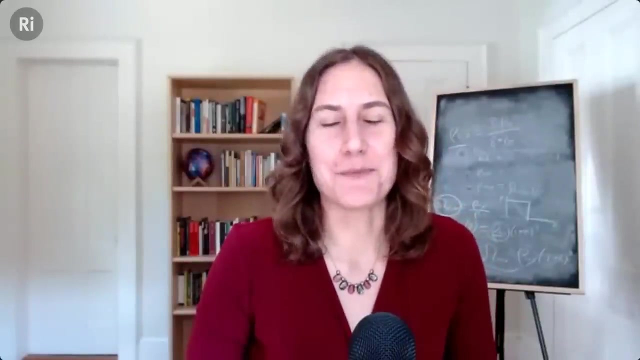 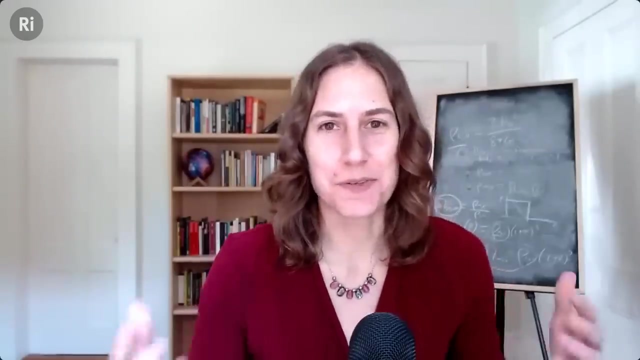 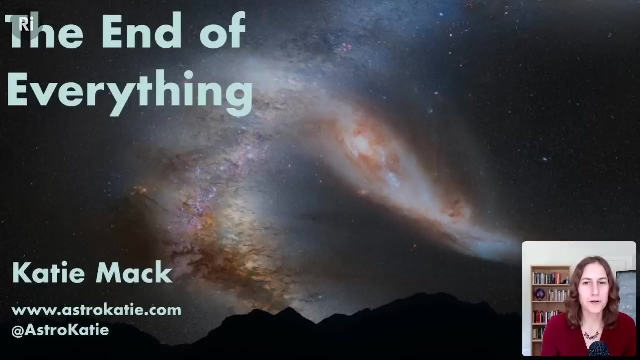 I am super thrilled to be here. I would be more thrilled to be there in person, but, times being what they are, this is still a wonderful opportunity to work with the Royal Institution and to give this presentation. So I'm super happy to talk with you about the end of the universe, the topic of my book, and in this presentation I'll be sort of walking you through a little bit about what we know about the cosmos and a little bit about how we think things are going to progress in the future. 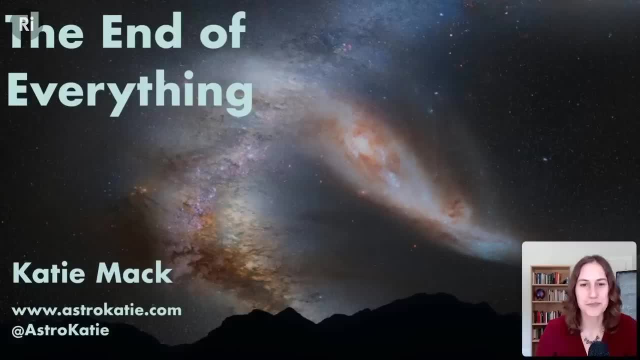 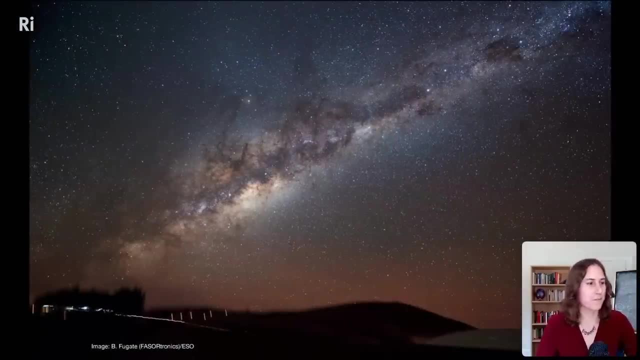 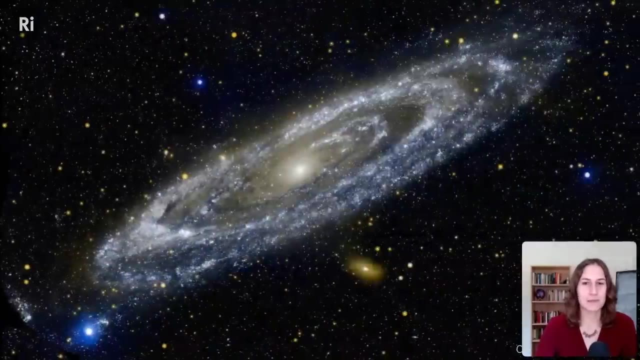 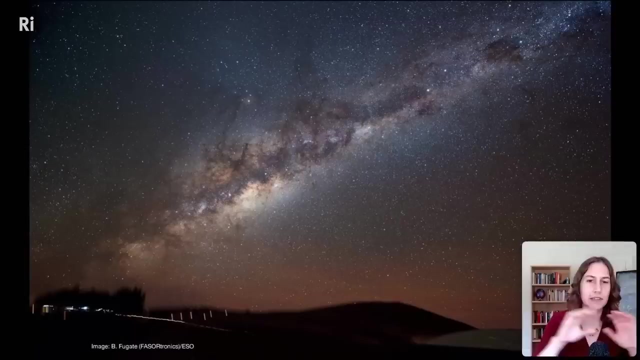 So yeah, without further ado, Without further ado, I will start things off. So we are here. We live on a planet inside the Milky Way galaxy. When we look out into the night sky, we can see this amazing, amazing band of stars across the sky, and those are the stars of the Milky Way galaxy. 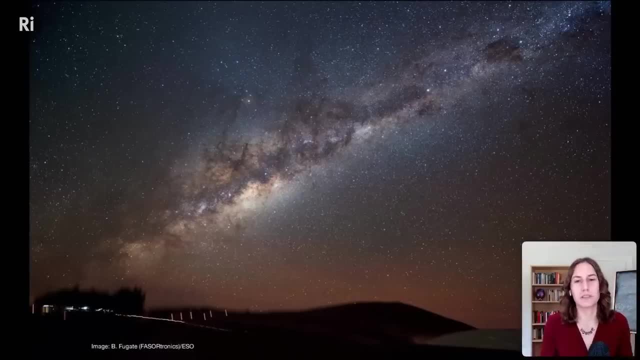 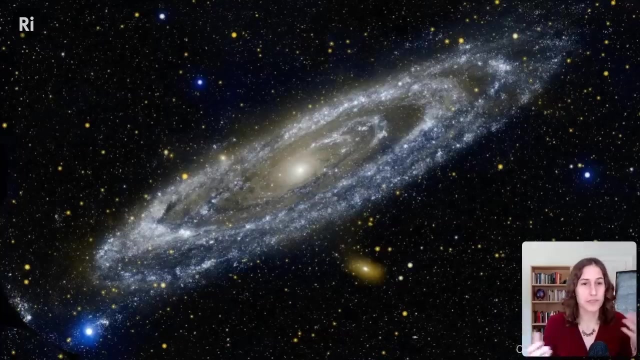 We have somewhere around 100 billion stars And if we were able to look out to look at our galaxy from the outside, it would look something like this: We would see spiral arms. We would see a bulge of stars at the center. 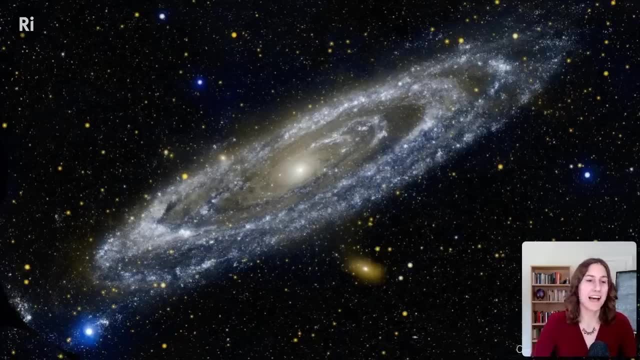 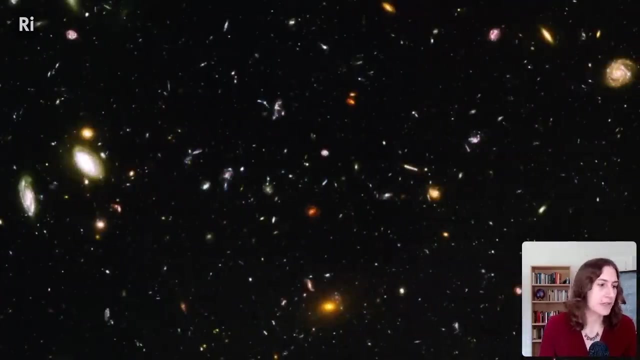 This is actually our nearest neighbor large galaxy, the Andromeda galaxy, And that will come up again later in the talk. But when we look out into the cosmos we see literally billions of stars. We see literally billions of other galaxies. This is a little piece of the Hubble ultra deep field. 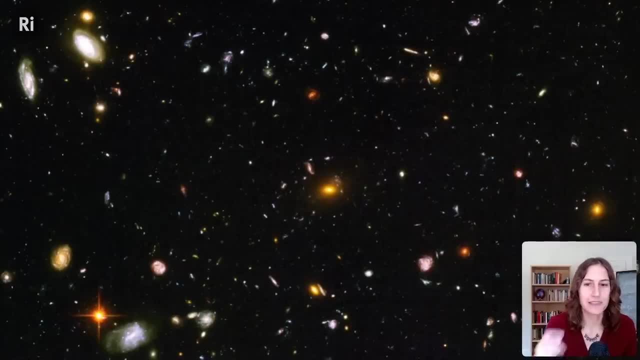 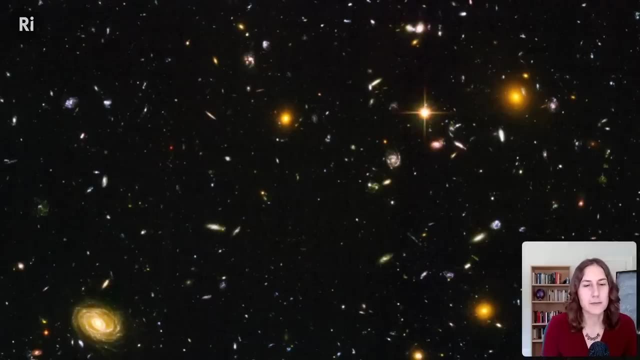 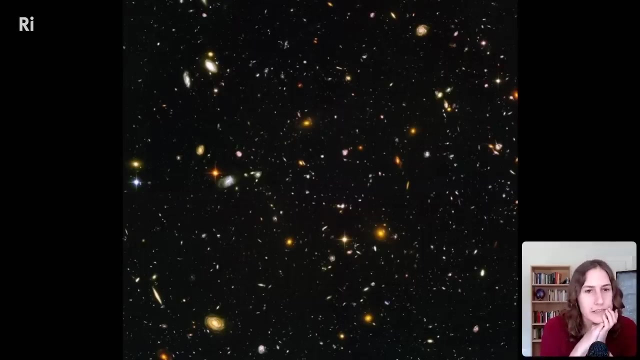 Just sort of panning through these, this image where this entire image contains something like 10,000 galaxies. in this picture right here, And when we look out into these images, we're seeing galaxies that are distant from us, Galaxies that are distant in the universe that are, in some cases, billions of light years away. 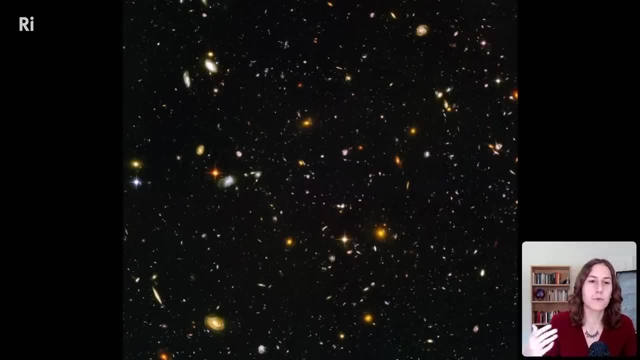 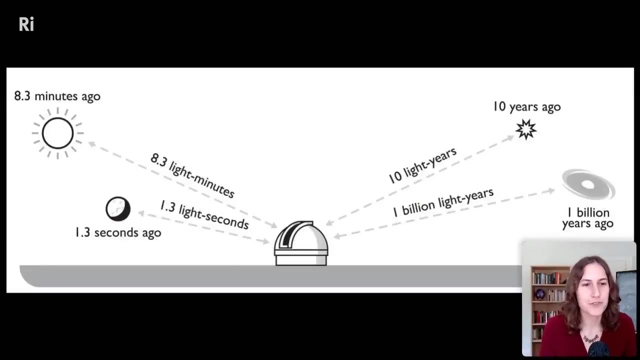 And because they're so far away, they're showing us light from the universe when it was younger In the universe. when we look at something distant, we're also looking back in time, because light takes time to travel to us. So if we are at an observatory on the earth and we look out at the moon, we're looking at 1.3 seconds ago. 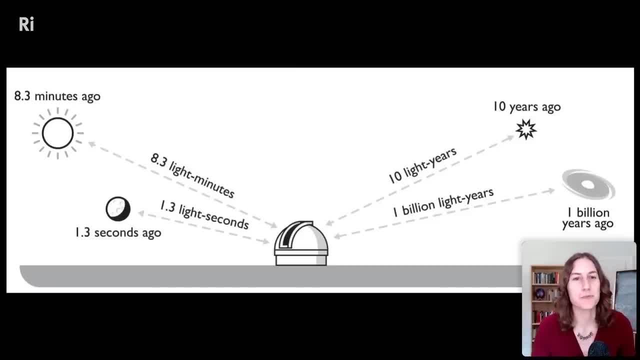 It's 1.3 light seconds away, Because it takes light 1.3 seconds to get to us. The sun is about 8.3 light minutes away, So it takes light 8.3 minutes to get to us. So we're looking at 8.3 minutes ago when we look at the sun. 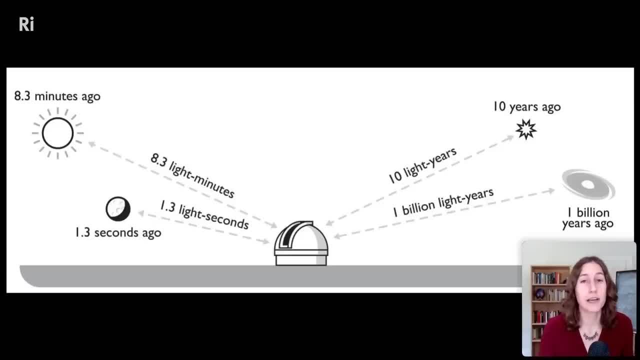 When we look at stars, we might be looking at many years ago, maybe thousands of years ago. When we look at other galaxies, we're often looking at billions of years ago, So we're really seeing the universe as it was in the past. when we look at something distant, 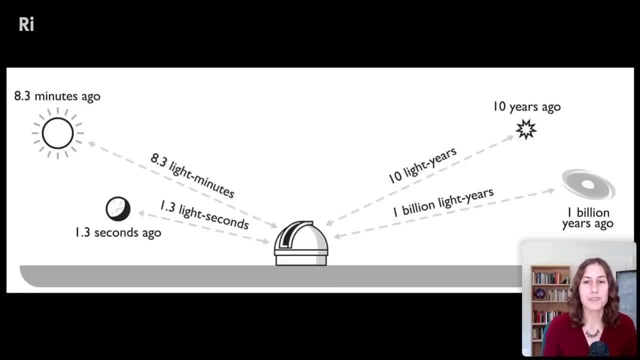 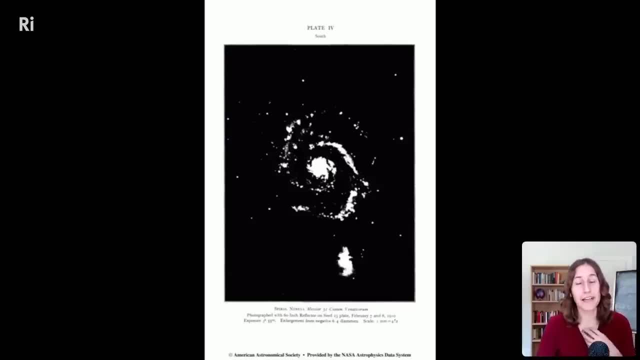 But we haven't always known what is out there, how distant it is, How distant things really are. In the past we didn't even know that there were other galaxies. It took a while to discover the existence of other galaxies, So for a long time astronomers saw these things called spiral nebulae, which were these collections of bright something in the sky. 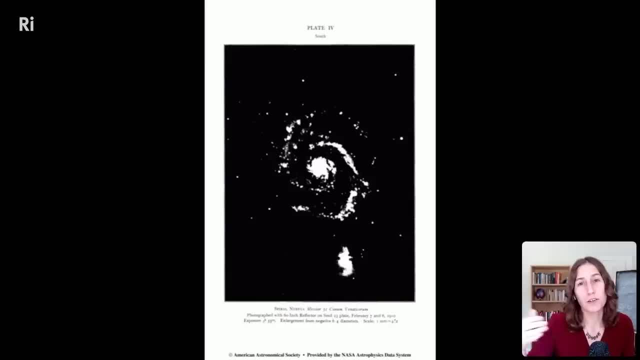 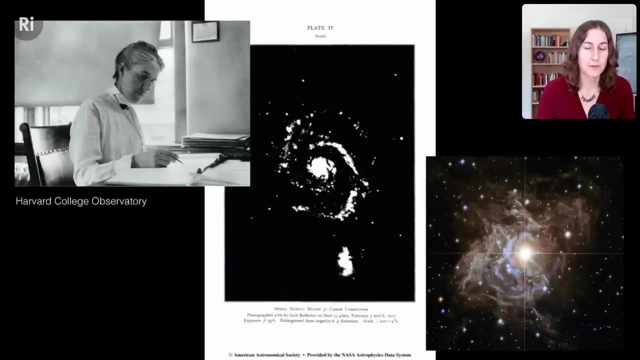 And the question was: are these parts of our own galaxy? Are they nebulae in our galaxy? Are there little collections of stars in our galaxy, Or are these very distant things, things like our own galaxy, but much farther away? And one of the ways that we were able to eventually figure out how distant these things were was due to the work of this person, Henrietta Swan Leavitt, who was working at the Harvard College Observatory. 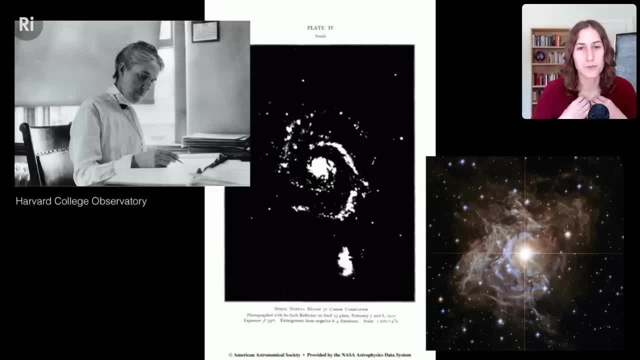 And she was looking at a certain kind of variable star called a Cepheid variable star, which you can see there in the corner of your screen. That's an example of these stars, And these are stars that brighten and dim in a particular pattern. 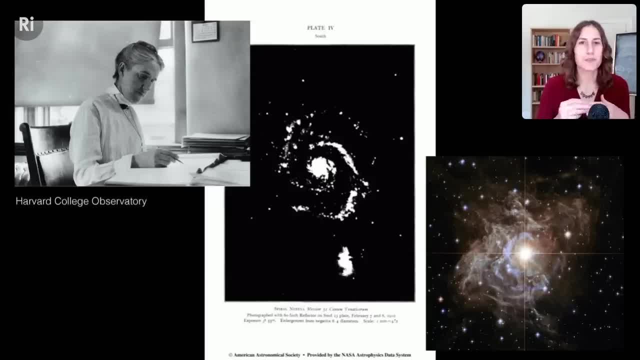 And because the brightening and dimming is related to how bright they are intrinsically, it was possible to use these as kind of mile markers in the universe and to look at some of these variable stars in nearby galaxies and see that these galaxies really were very, very distant and outside our own galaxy. 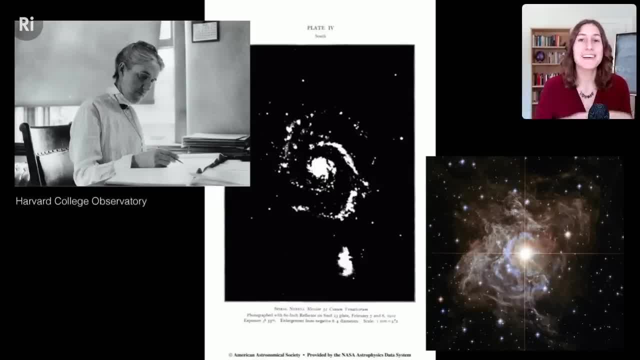 So by seeing these variable stars in nearby galaxies, we were able to see that these galaxies really were very, very distant and outside our own galaxy. So by seeing these variable stars in the spiral nebula, that gave us a impression of the size of the universe, of how far away these galaxies were. 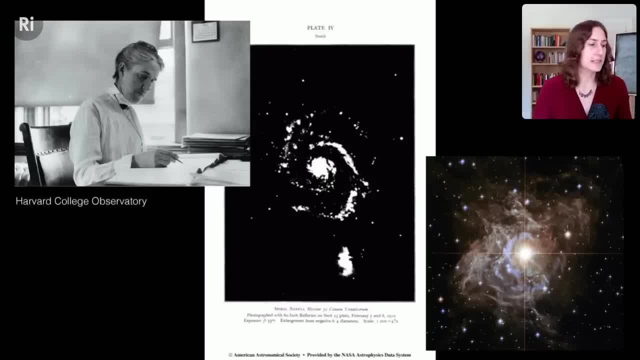 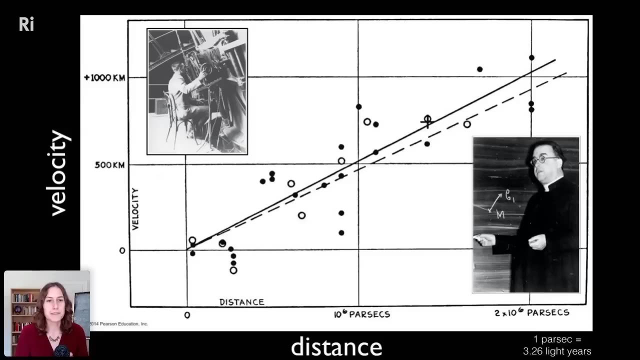 And once we knew that these galaxies were very distant, we were able to then learn something about how they were distributed in the universe and also how they were moving in the universe. So in the 1920s, these two people were responsible for figuring out where they needed to be. 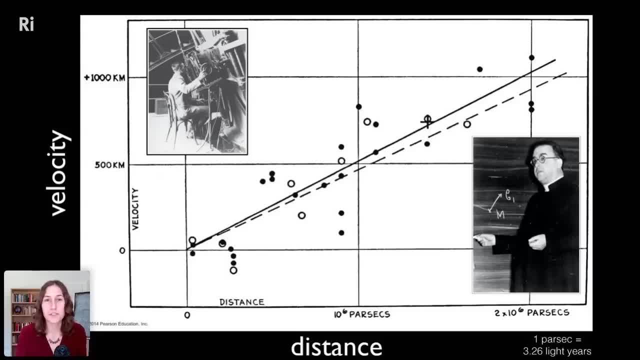 that the universe is expanding. They contributed in different ways. So on the upper left there, that's Edwin Hubble, And this diagram is a diagram that he put together in a paper where he was showing that, as you go to farther and farther distances, the speed at which galaxies appear, 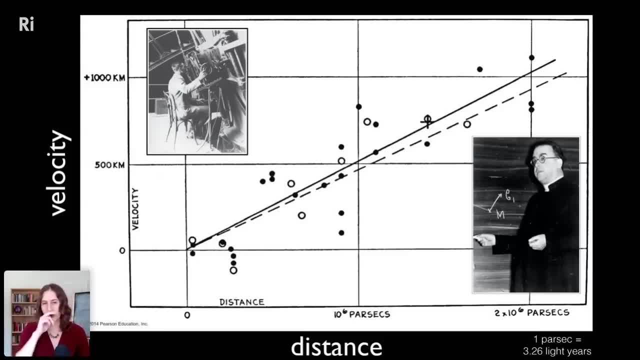 to be moving away from us is increasing, And the person in the bottom right corner of your screen there, that's Georges Lemaitre. He was a theorist. He was thinking about how the universe has been evolving over time And he worked out that in a universe where the universe is expanding, 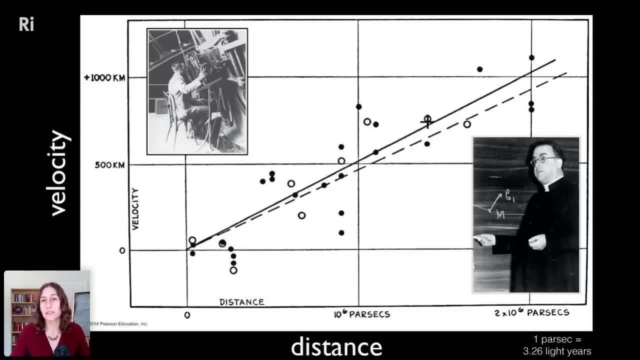 it would look like all the galaxies are moving away from us. It would look like every galaxy is moving away from every other galaxy. And he used that reasoning to decide. well, maybe this means that the universe was smaller in the past and has been increasing, And maybe 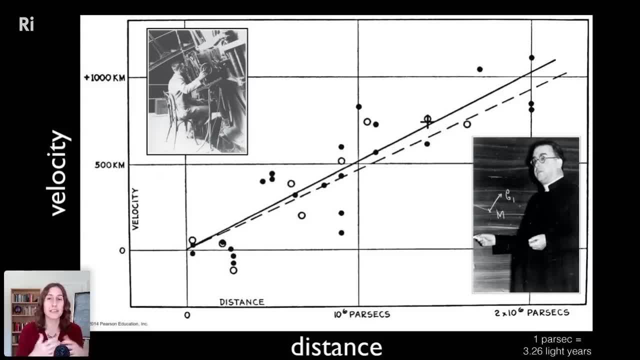 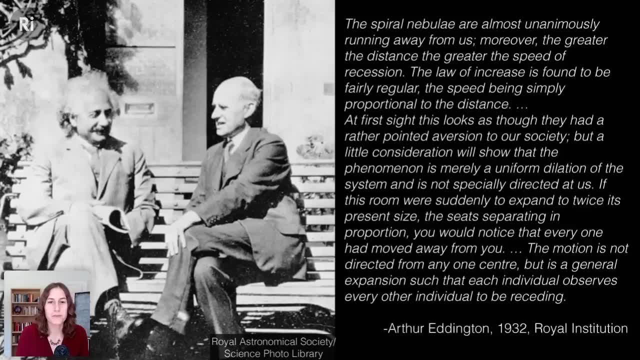 there was a change in the universe. Maybe there was a change in the universe in the past. There was a time when the universe was very small And that kind of led to the idea of the Big Bang. So once it was determined that distant galaxies were moving away from us, there was a discussion. 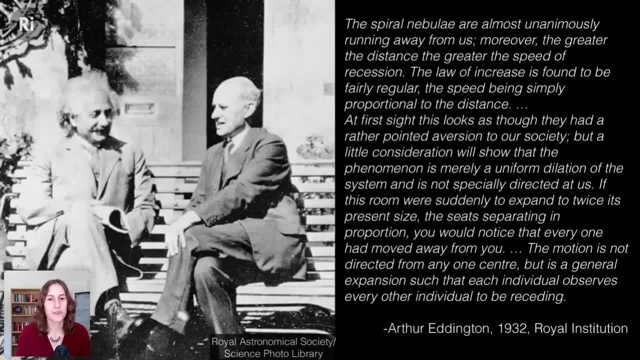 about what that means for the universe, And one of the people who expressed that very well at a lecture at the Royal Institution in the 1930s was Arthur Eddington. He's probably most famous for taking some observations that helped confirm Einstein's theory of relativity, And you can see him. 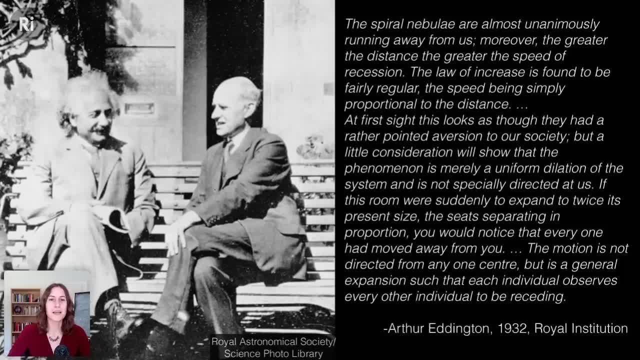 here in this image, sitting with his colleague Albert Einstein, But I like the way that he talked about the way that galaxies are moving away from us. He says: the spiral and nebulae are almost unanimously running away from us. Moreover, the greater the 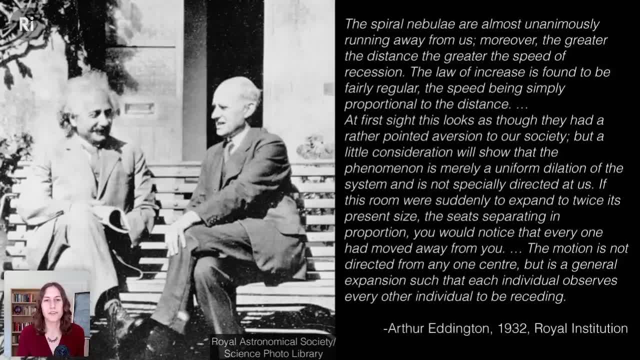 distance, the greater the speed of recession. The law of increase is found to be fairly regular, speed simply being proportional to the distance. At first sight, this looks as though they had a rather pointed aversion to our society. But a little consideration. 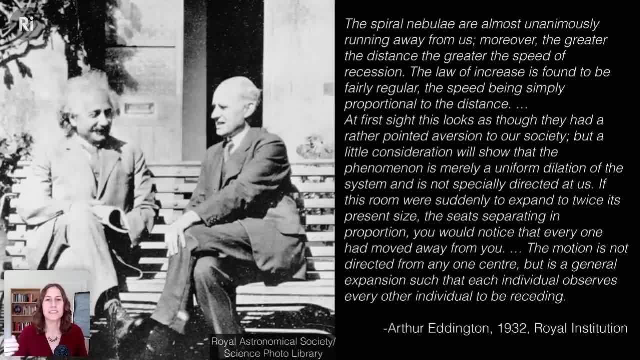 will show that the phenomenon is merely a uniform dilation of the system. It is not specially directed at us. If this room were suddenly to expand twice its present size, the seats separating in proportion, you would notice that everyone had moved away from you. The motion is not directed. 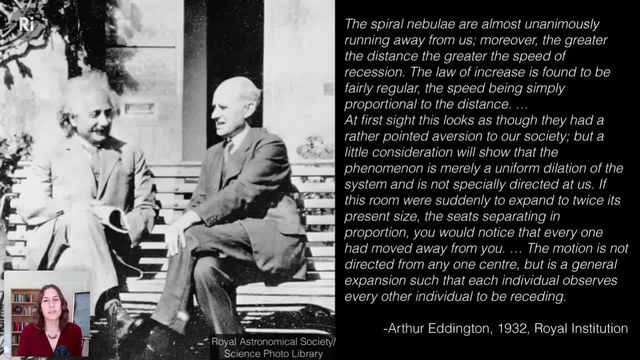 from any one center but is a general expansion such that each individual observes every other individual to be receding. And that's a really important point, that the expansion of the universe is not the expansion from a center point, It's the expansion of the entire universe in every 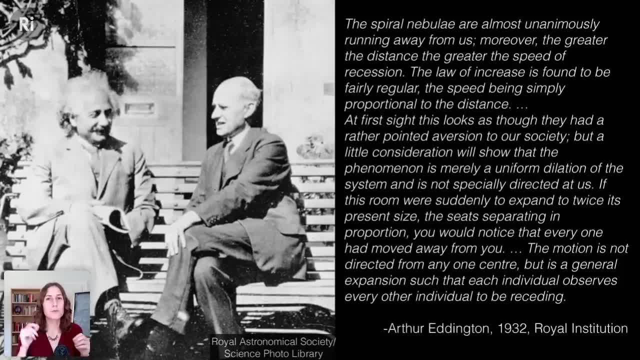 direction at every point, And so there's no center from which we're expanding. The whole cosmos is getting bigger. The whole cosmos may have always been infinite in size, and it's just getting more infinite as it expands. It's a strange concept to keep in your mind, but really what we see is just 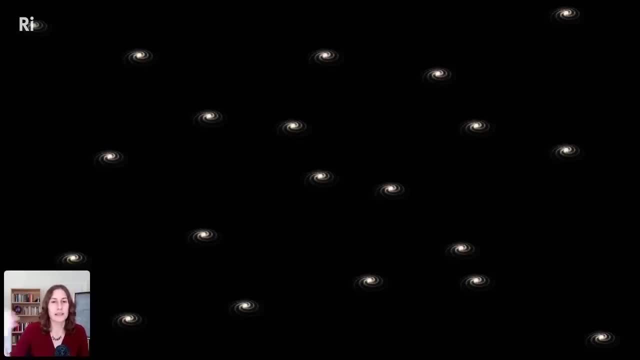 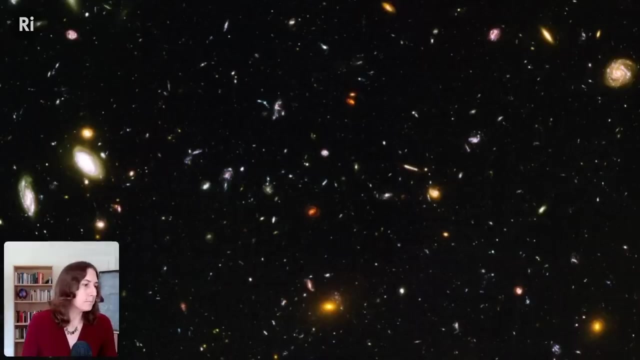 that things are getting farther apart. So if we look at the distribution of galaxies in the universe and we kind of move forward in time in our picture of this, we see that galaxies are getting farther and farther away from each other as time goes on. And so when we look at some of these distant galaxies that are 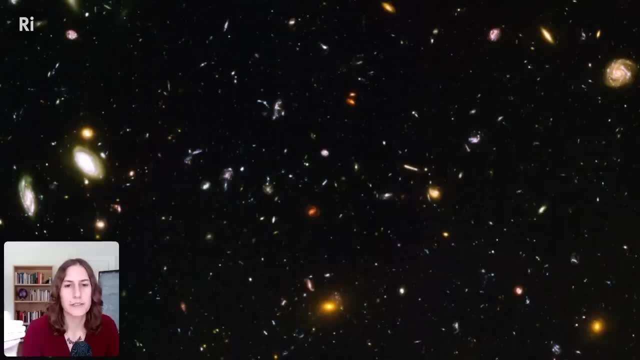 moving away from us very quickly and we're looking far into the distance. we're also looking far into the past, And we can look so far into the past, so far into the distance. we see these rapidly receding galaxies. We see them as they were. 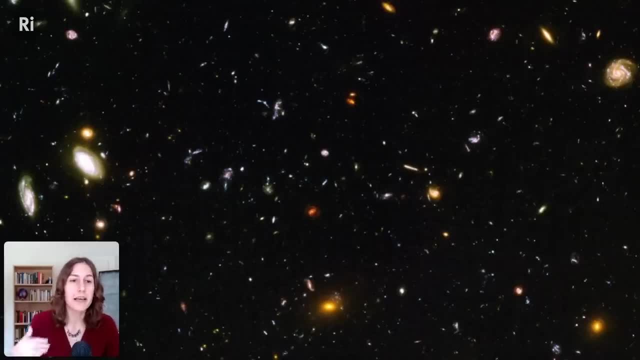 When the universe was very young, because they're so far away, And so there are kind of two things that we can get from these kinds of ideas: that the universe is expanding. galaxies are moving away from us. We see very distant ones when the universe was young. What that can tell us is that 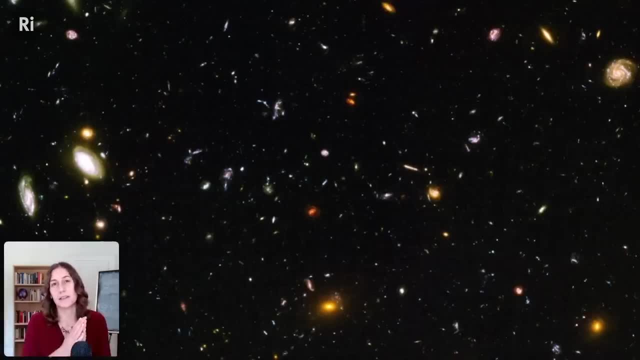 in the past the universe was much more compressed that the universe has been expanding over time. So in the past it must have been smaller, It must have been denser, It must have been hotter, because everything was closer together, because everything's closer together. 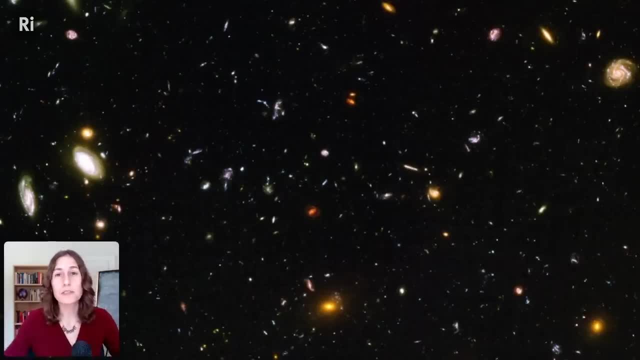 It's compressed, And when we look into the cosmos in the distance, we should see parts of the universe that, from our perspective, are earlier in the cosmos, in a cosmos that was smaller and hotter and denser, And so we can map out what that sort of would look like. 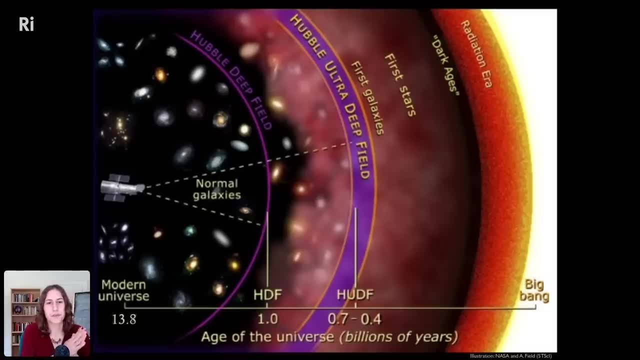 And we can say that. you know, our current universe is about 13.8 billion years old And we can use telescopes like the Hubble Space Telescope to see distant galaxies. So in this image, this purple band is the Hubble Ultra Deep Field. That's that image I showed you before. 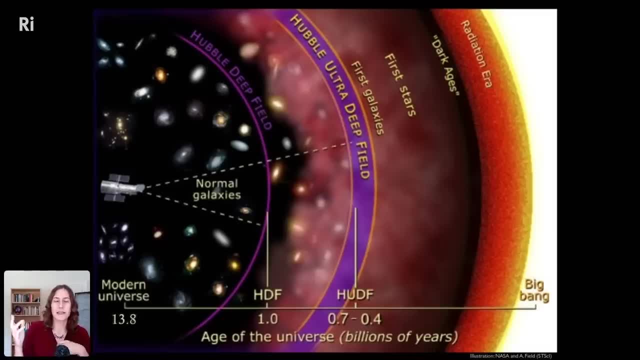 with the 10,000 galaxies in it. Those galaxies are so far away that they're mostly living at a time when the universe was about half a billion years old. So when we look at those galaxies, we're looking at a half a billion-year-old universe rather than our own 13.8 billion-year-old universe. 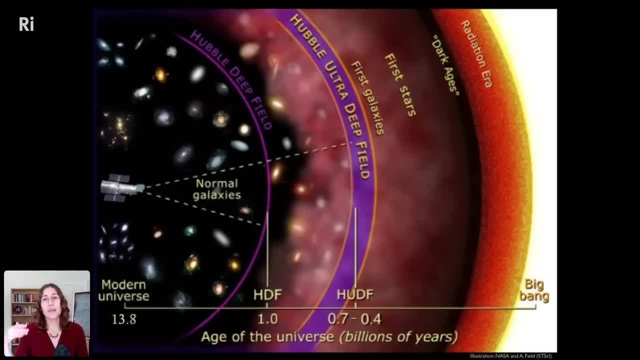 But in principle we can look beyond that And we can see times when their galaxies didn't exist yet, when the universe was just hot and dense everywhere, Because in the beginning the universe was hot and dense everywhere. The Big Bang was a time when the universe was hot and dense everywhere And 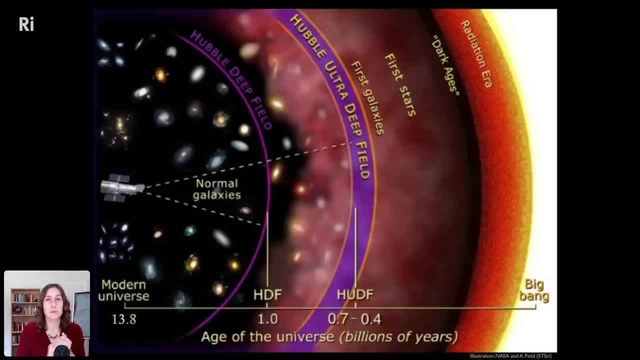 if you just dial back the expansion, you get the idea that there was a time when the whole universe was sort of filled with this fiery plasma And it was everywhere, because there's no center to this expansion. Every part of the universe was filled with this hot plasma in the early days And the 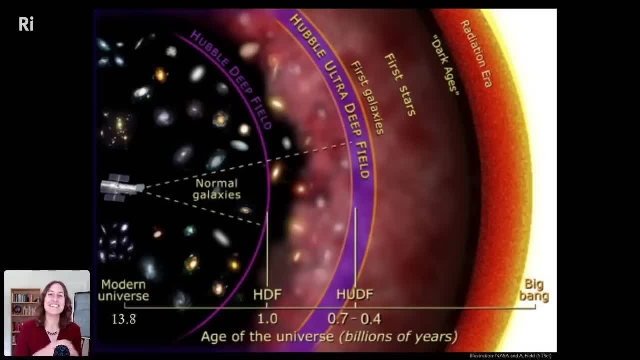 universe is held onto this plasma. And so far away we can see a lot of that plasma. and so far away we can see the plasma. And so far away we can see the plasma. And so far away we can see the plasma. There was the first cosmic layer in the universe. And so far back in the 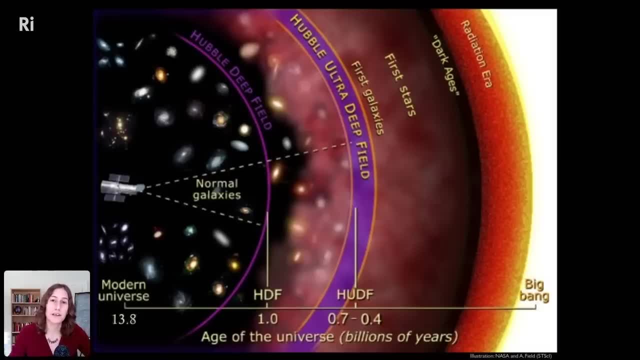 early, I mean, there weren't days yet, in the earliest moments of the cosmos, And so we should be able to see in every direction. if we look far enough, We should see that hot, dense plasma. We should see the light from the glowing of that plasma before the universe cooled and expanded. enough for that fire to kind of calm down and go out. And we do see that Some of the first people to observe that were the guys, Pensias and Wilson, who used a gas- Journalist. They used a gas, gas, gas, gas. 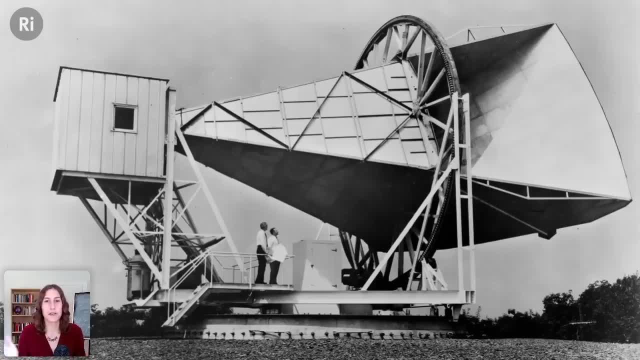 were these two guys, Penzias and Wilson, who used a microwave receiver to examine the sky and they saw this sort of background static in the receiver and they tried lots of ways to try to figure out what this static was and it turned out that this static 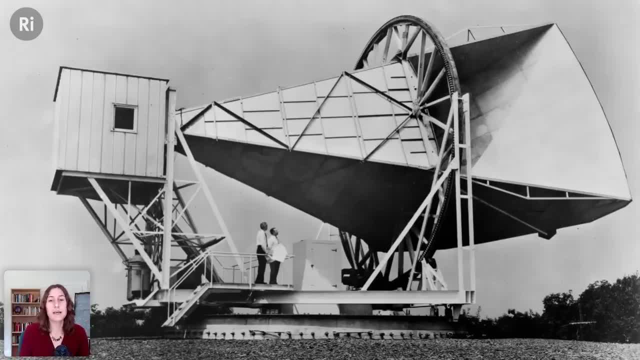 that they were getting in their receiver that was coming from every direction in the sky was actually this background light from the Big Bang. They were seeing parts of the universe that, from our perspective, were still on fire, and those parts of the universe, those very, very distant parts of the universe. 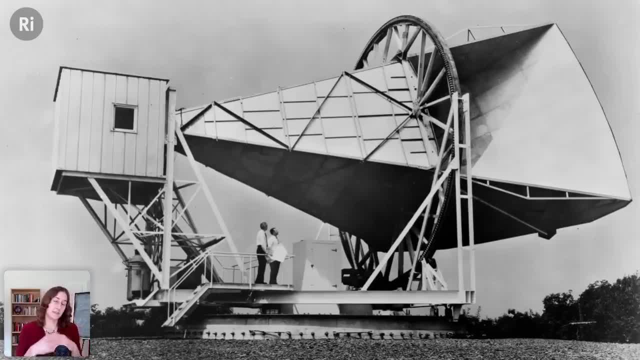 were emitting this radiation, this microwave radiation that looks the same in every direction. So they were able to. you can take that radiation. you can map out what it looks like on the sky, so just like you can take a map of our whole sky in visible light. 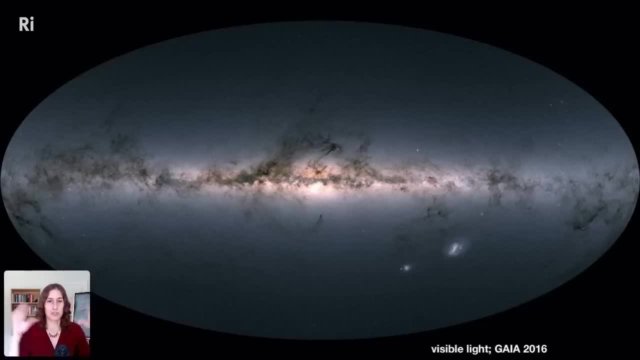 this is a map of the galaxy in visible light stretched out so you can see the whole sky in one image. so this is a projection of the whole sphere around us as an oval. You can do that with visible light and if you do that, with microwave light. 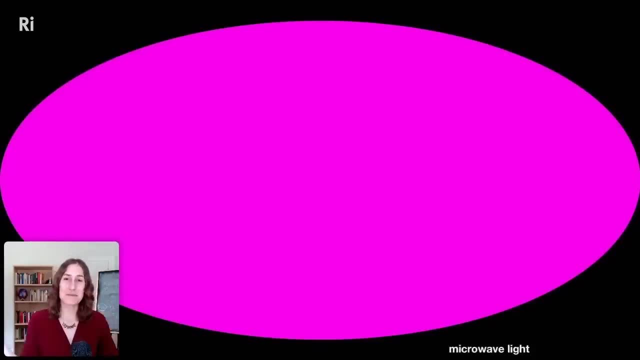 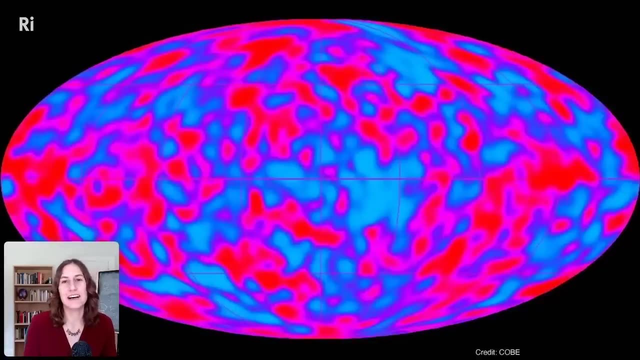 it's very boring. actually It just looks like the same color of microwave light in every direction, but if you crank up the contrast a little bit you can start to see variations on that background light and you can see parts of the background light that were a little bit hotter. 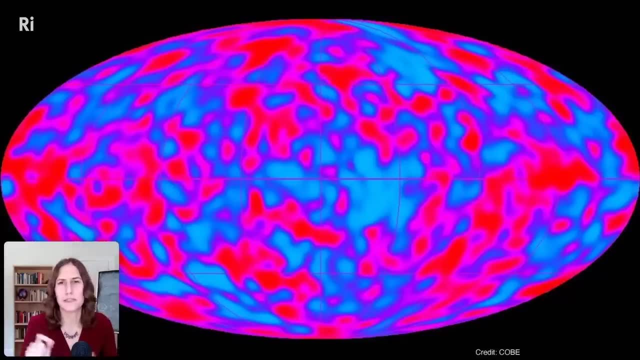 or parts that were a little bit colder, and this is one part in 100,000.. These are very small variations. You have to crank up the contrast a lot to see them, but what you're seeing is that background light, that light from when the universe was still on fire. 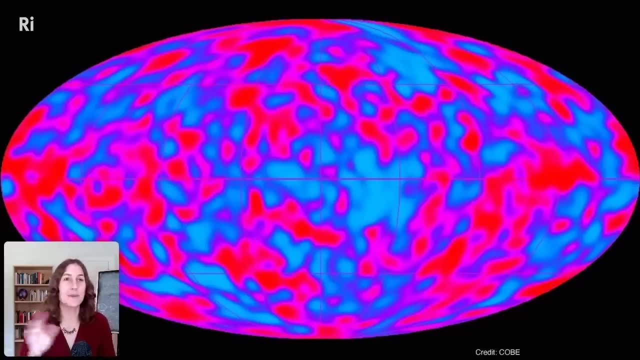 and there are ways that we know that that's what we're seeing, but it's not some other kind of weird signal in the universe, because we can take the spectrum of that light. We can analyze how that light is distributed along different colors of microwave light. 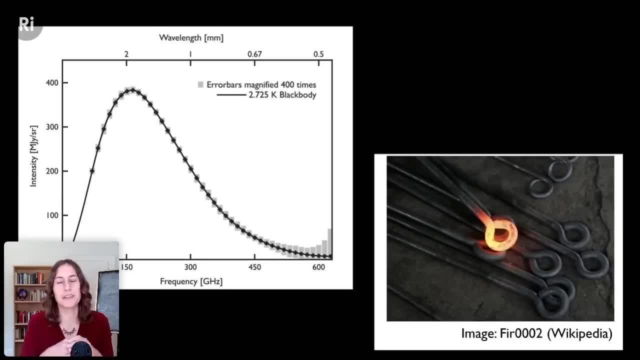 and we can see that the shape of the spectrum, the distribution of energy across different frequencies of microwave radiation, is the kind of shape that you get when you see something that's just glowing with heat. This is called a blackbody spectrum. It's a way that the energy distributes itself. 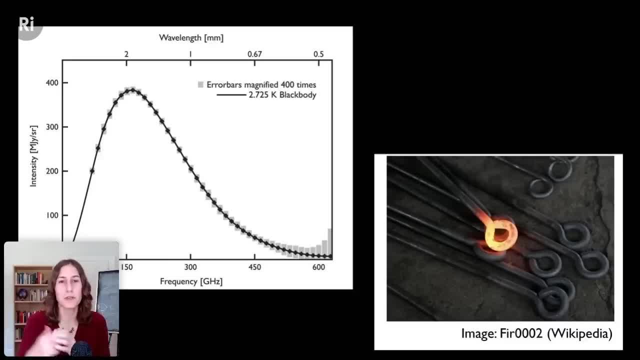 If you just heat something up and watch it glow, so the same way that if you take a poker and put it in the fire and let it glow red hot that the spectrum of that light would make this blackbody curve this particular distribution of radiation. and when we look at the microwave, 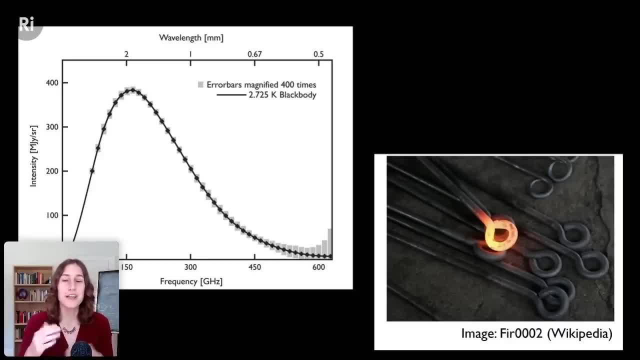 background radiation, this background light from the early universe. it's exactly that shape. I mean. it's such a perfect fit to this spectrum that you get from things that are glowing because they're hot that you can't even see the errors in the measurement unless you magnify them 400 times. 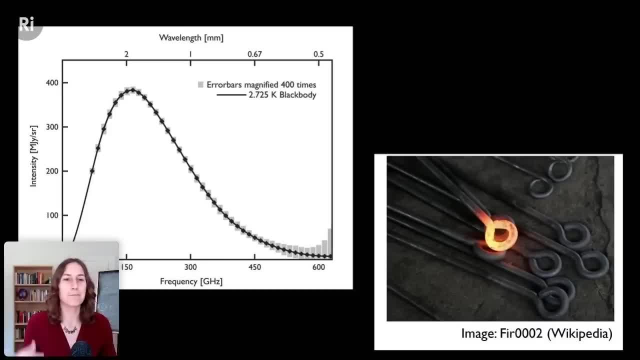 like in this diagram that I have here, where you can actually see the uncertainties in the measurements, because we've magnified them. It's the most perfect blackbody spectrum ever measured, which means that light we get from the background light of the universe really is just the universe glowing. 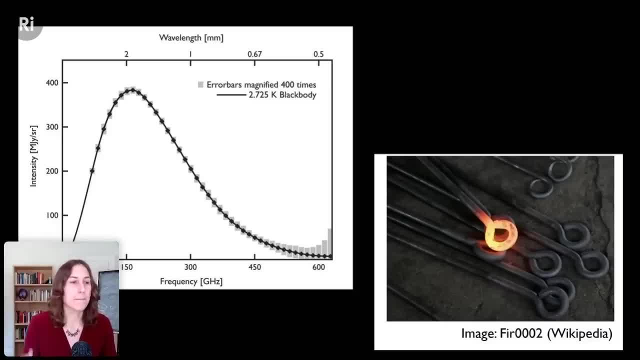 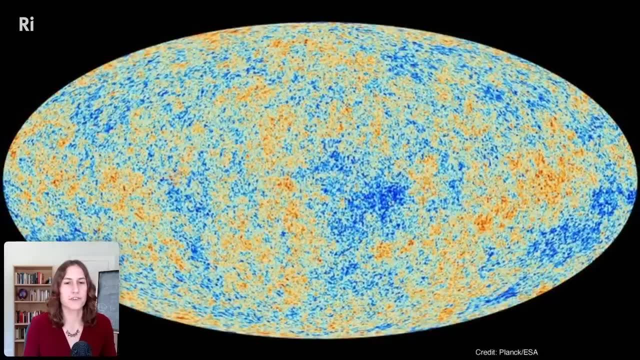 because it was hot. It's an amazing thing and we can crank up the contrast some more on this image. We can look at smaller variations and smaller variations, and we can see this detail where we see little bits of the universe that were a little bit hotter. 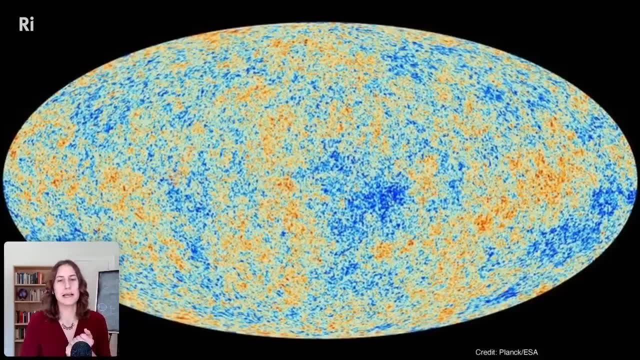 or a little bit cooler, a little bit more dense, a little bit less dense- in the earliest days of the universe. It's somewhere around 380,000 years after the very beginning, whenever the very beginning was, and 380,000 years might sound like a long time. 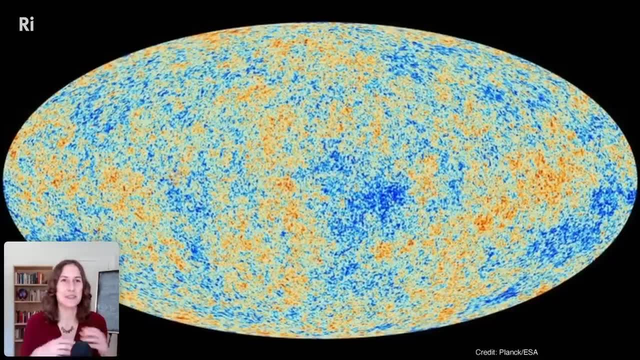 but compared to 13.8 billion years it really isn't. It took 380,000 years for that primordial fire to cool down and to dissipate enough that light could kind of travel freely through the universe and not just be in this glowing space. 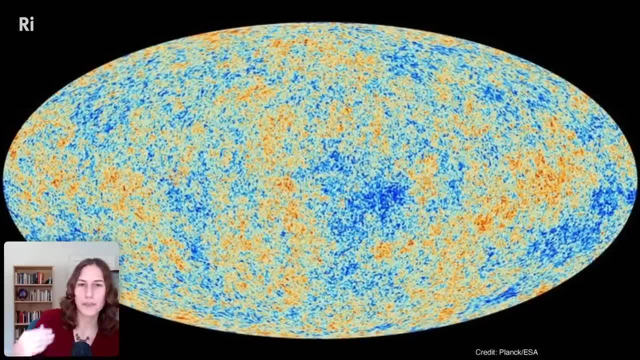 and so we can use that background light, We can use the little variations in it to learn about what the universe is made of, about how it's been evolving over time, and we can start to learn something about the possible future of the cosmos through looking at this light. 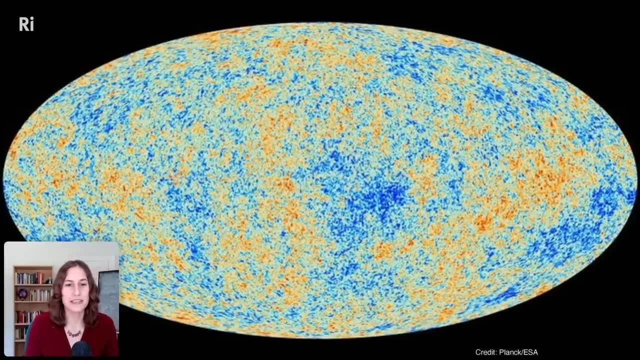 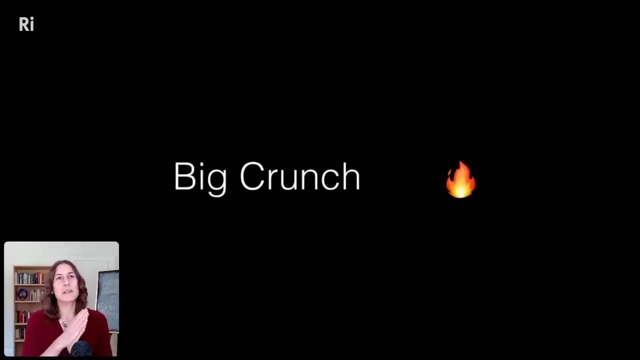 and examining what we see in this background light, and that brings me to discussing the first possibility for the end of the universe, which is the big crunch. Now, the big crunch is an idea that's been around for a while, and it's the one that was thought to be most likely. around the time when the microwave background light was first discovered, and the way the big crunch works is okay. right now, the universe is expanding. Galaxies are getting farther apart from each other. That's the expansion that was kicked off by the Big Bang. but as the galaxies are moving apart from each other, there's still gravity between each of these galaxies, and all the gravity of all the stuff in the universe should be trying to kind of slow down that expansion. All the gravity is trying to pull everything back. 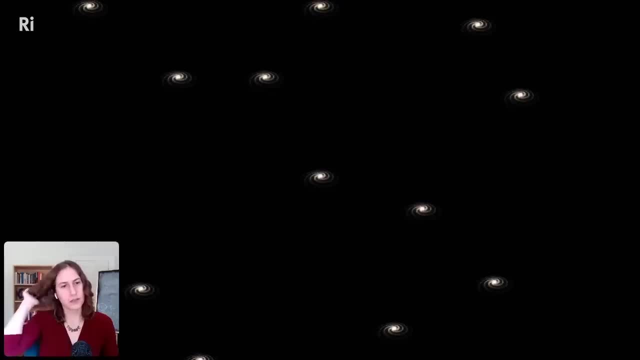 and so there was a debate from the 1960s to the late 1990s about whether the expansion would keep going forever or whether at some point the expansion would reverse and galaxies would start coming back and you know, the whole universe is sort of sort of collapsing. 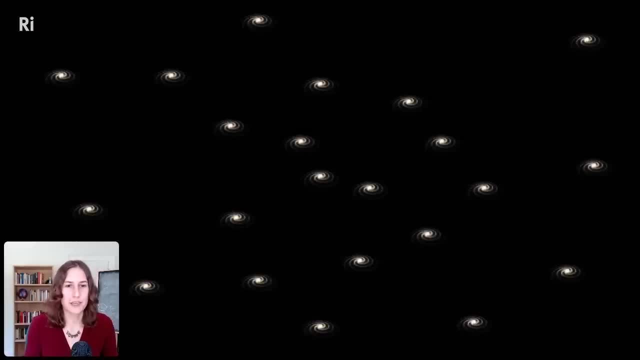 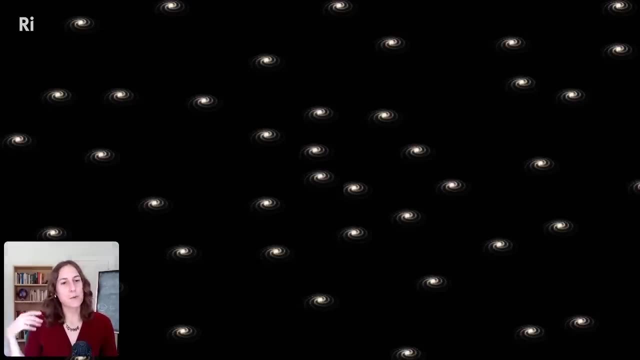 into a smaller and smaller space and sort of reversing the expansion of the Big Bang and bringing everything back together again. Now we think it probably won't come back together again, but let's just take a moment to talk about what it would look like if it did. 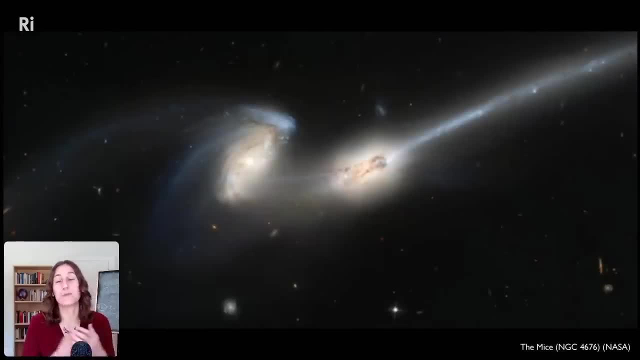 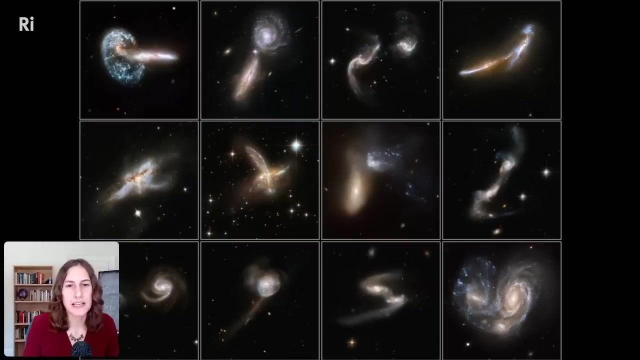 so the first thing that would happen is that galaxies would start to collide with each other. They would be interacting with each other and, as when galaxies collide, they sort of come together, the stars within the galaxies get flung out in these long trails and we see, we see galaxy collisions all over the universe. 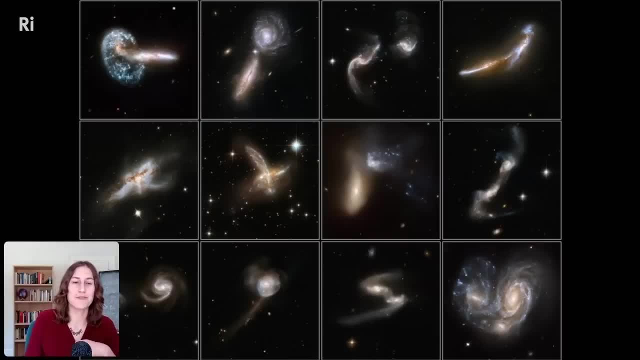 and this is just a sample of some interacting galaxies that have been seen by our telescopes, and you can see these, these amazing tendrils of stars, and one of the things that happens when galaxies collide is that the the gas, when it comes together in these these different galaxies, the gas comes together and 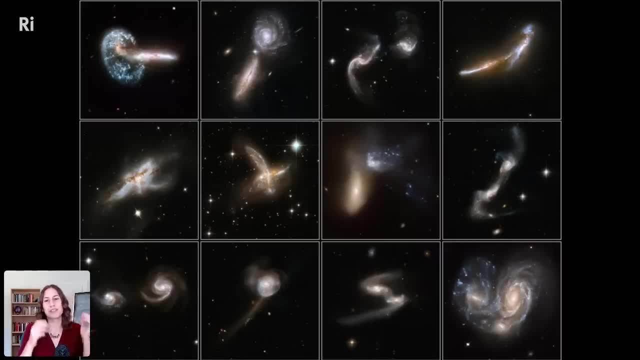 creates bursts of new star formation. you get black holes colliding and the black holes are out, putting out, you know, jets of radiation and there's all sorts of amazing. it's kind of an amazing light show that happens when galaxies collide. what doesn't happen generally is it doesn't happen that the individual stars. 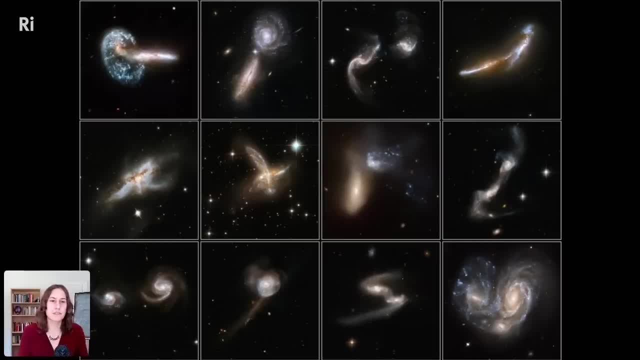 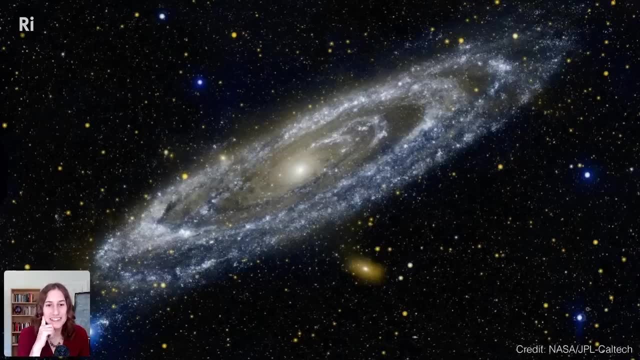 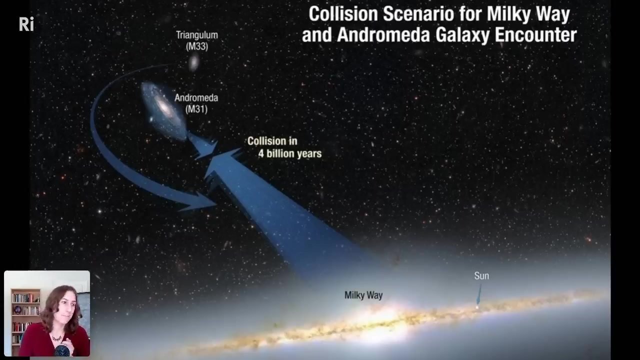 because of this. so this is the Andromeda galaxy I showed a picture of before, our nearest neighbor, large galaxy, and it is coming toward us. it is coming for us at about 110 kilometers a second and in about four billion years the Milky Way and the Andromeda galaxy will collide with each other, and that'll be really 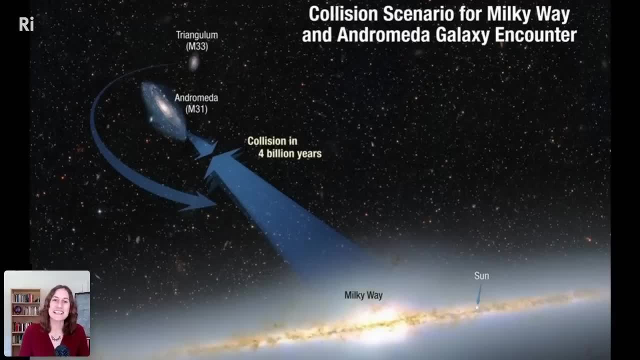 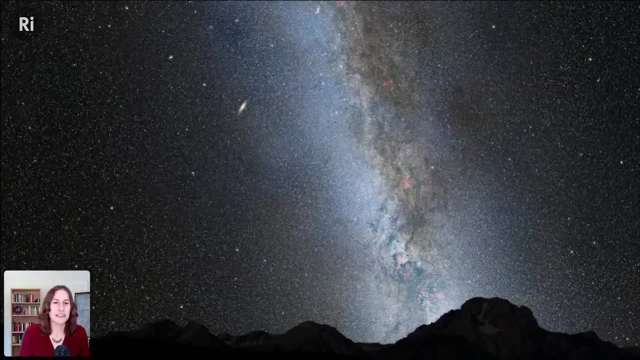 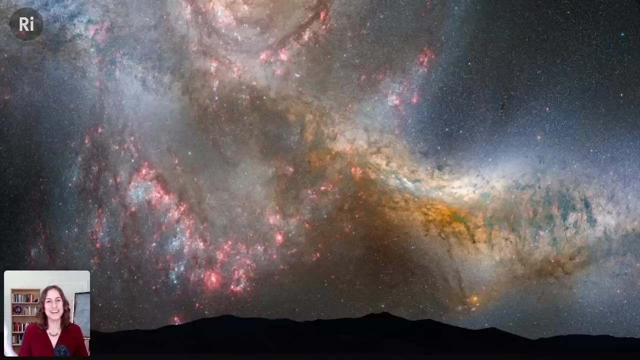 cool to see if, if anything is left in the in our solar system to to watch it, we will see the Andromeda galaxy starting to get larger on the sky as it as it approaches and oh no, it will- it will smash into the Milky Way move. 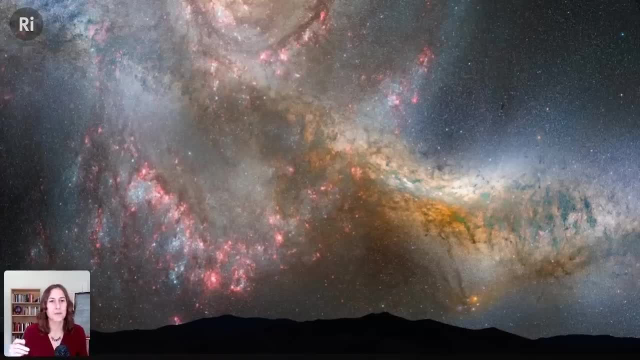 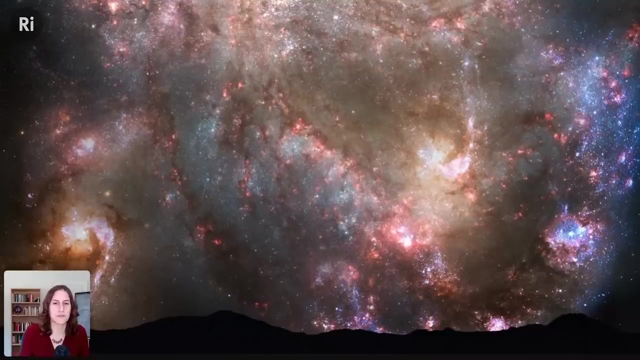 stars around. in this image you can see little clumps of blue and red where stars are forming and going supernova. you can see these dust trails as as as stars are going supernovae and creating dust out, pushing dust out into the universe, into the collided, collided galaxy, though. 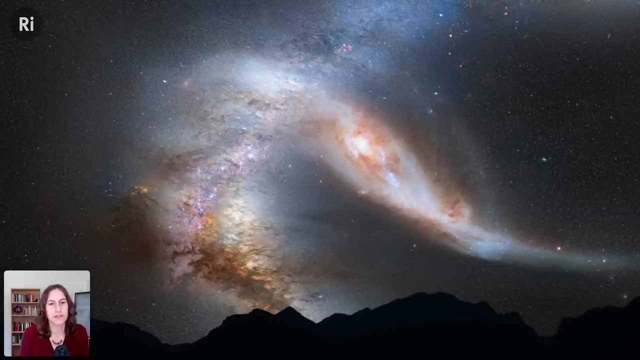 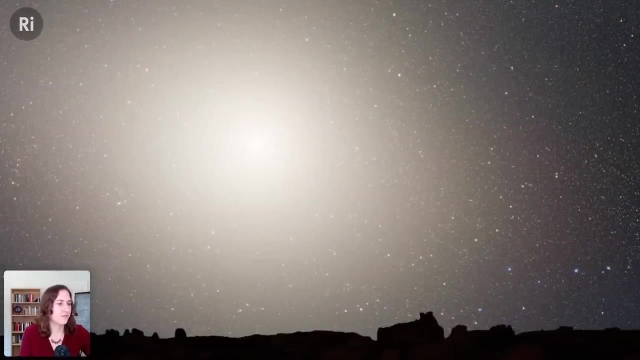 it'll kind of go through more than one pass and stretch out the, the Milky Way and the Andromeda galaxy and over time it'll settle into a kind of as final state of this sort of elliptical collection of stars where the star formation will have settled down and and you'll just get these, these old. 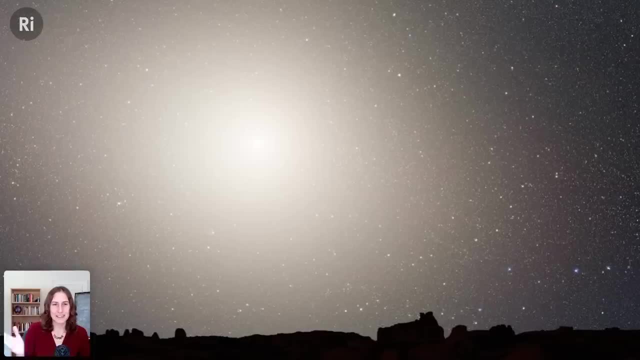 stars hanging out and and slowly evolving over time. so we're gonna see that up close, or whatever's left of our solar system, we'll see that up close. of course, by four billion years from now, the Sun will have expanded quite a bit. we'll be moving toward its red giant- red giant phase. it will have swallowed up. 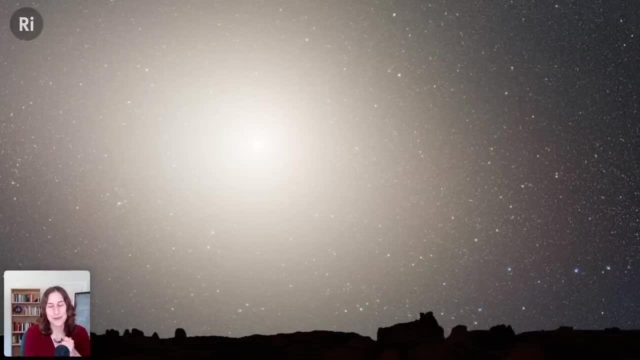 Mercury and Venus and might be might be destroying Earth by then. so probably we won't be around to watch it, but maybe we'll leave some little webcam going so we can see the see. you see the light show as we, as we've moved onto somewhere else in the universe. but the point is that that these kinds of collisions with 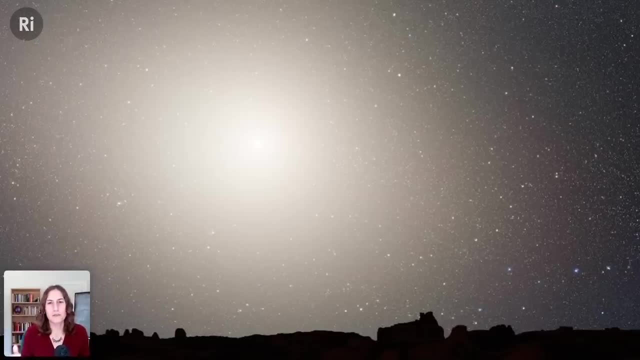 galaxies don't necessarily disturb, don't necessarily affect the stars of the solar systems per se. when galaxies collide, the chance of two stars hitting each other is minimal and so generally you know, there's just so much space between stars that that you know, more or less stars and solar systems will be okay. when, when the universe gets very dense, in a collapsing universe, the thing that kills the stars is not the matter but the radiation. so I mentioned that there's this, this radiation throughout the universe from the Big Bang, this leftover light from the, the afterglow of the Big Bang, and that light is just kind. 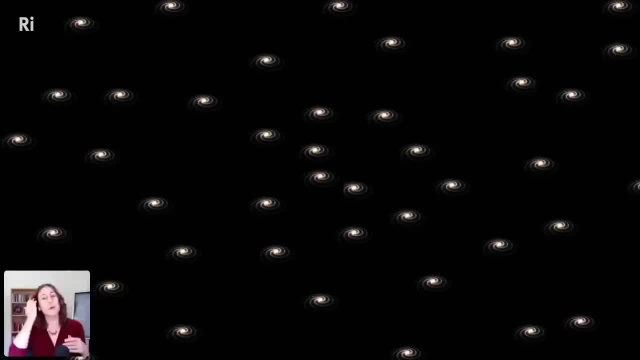 of out there traveling across the universe and we're picking some of it up. when the universe is collapsing, that light will become more condensed and it'll be like moving back toward that time when the unit, the whole universe, was full of this, this hot radiation. but it's not just that. ever since stars 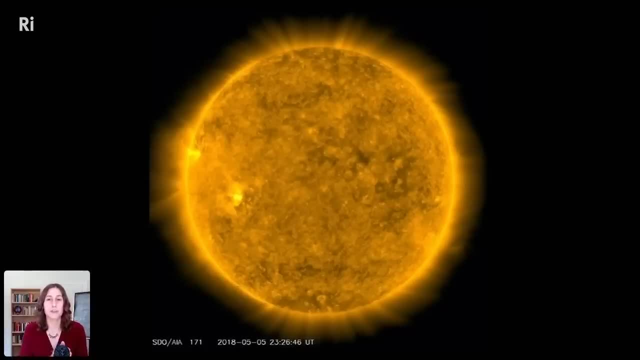 first formed in the universe. they've been putting out their own light, their own radiation, and when the universe is starting to collapse, that radiation, that light, will also become condensed and it'll be. it'll be moved to hotter parts of the spectrum. it'll be more, become more energetic light and as that light, 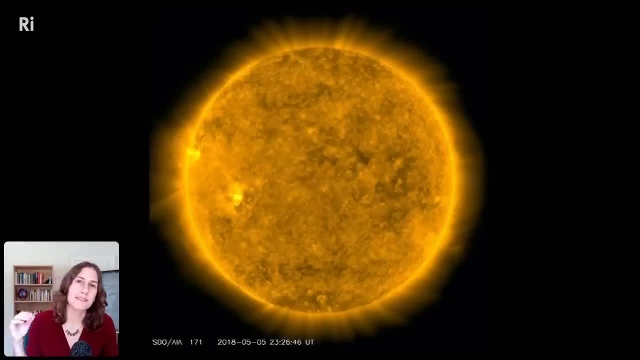 is compressed. that's what kills the stars. what happens is that, as the light is compressed- that's what kills the stars- is that that radiation, that hot, intense, hard radiation, is going to be so hot just through all of empty space that it will start to actually ignite the surfaces of stars, and at that point you know, nothing can survive. when, when you have thermonuclear explosions happening across the surfaces of stars, everything's toast. so so the big crunch would be a very, a very unpleasant thing to live through. now we're pretty sure that's not going to happen. uh, the thing that's, that's most. 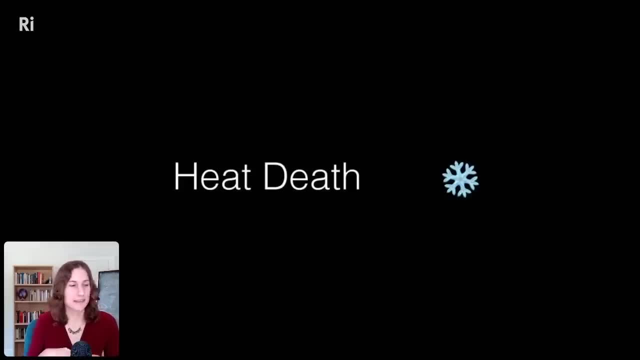 likely if you ask, Ask Cosmologists, is is called the heat death. now, the heat death starts the same way as the big crunch. the universe is expanding, galaxies are getting farther apart from each other and um, I mentioned that there was a time when there was a debate about whether the expansion would keep going forever or 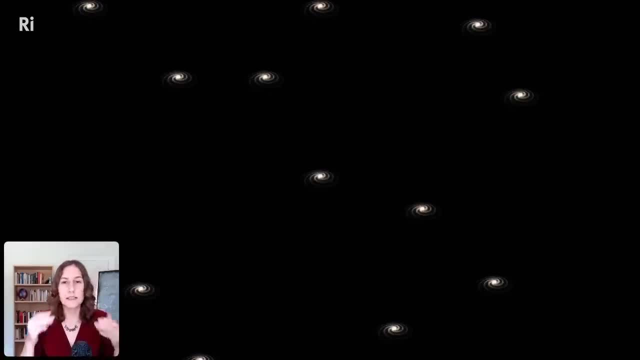 turn around and come back and in the late 1990s astronomers were trying to work this out. we're stopping the expansion of the universe and trying to see how much the expansion was slowing down, because the idea is that the gravity of everything in the universe should be slowing. down the expansion that was kicked off by the Big Bang. Just like if you throw a ball up into the air, the gravity of the earth slows down the ball in its ascent. At some point the ball will stop and fall down, unless you can throw 11.2 kilometers. 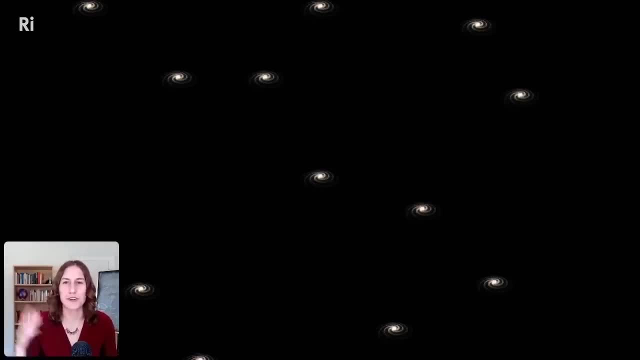 per second, and then it might escape out into the cosmos and keep going forever. So the question was: will the universe keep going forever like a ball that's thrown at the escape velocity of the earth where it just barely sort of reaches, you know, gets? 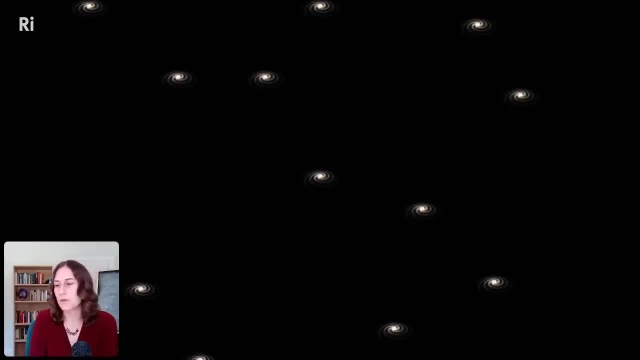 out of the atmosphere and then sort of coasts forever, Or will the ball come back? Will the universe re-collapse? And when that measurement was made, the surprising thing was that actually neither of those answers were true. The deceleration everyone was trying to measure turned out to be a negative number. 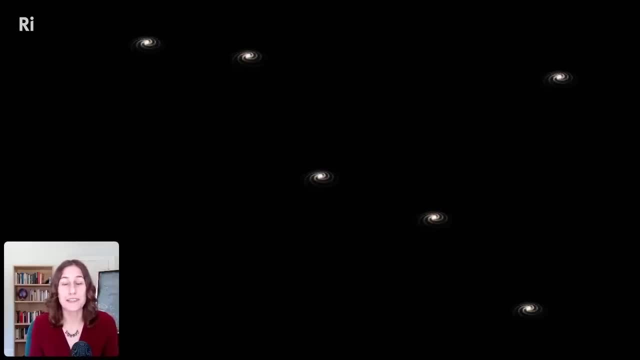 The universe was not decelerating, it was actually speeding up in its expansion. The universe was expanding faster and faster And that's very strange. That's about as strange as if you throw the ball up in the air. it slows down for a little. 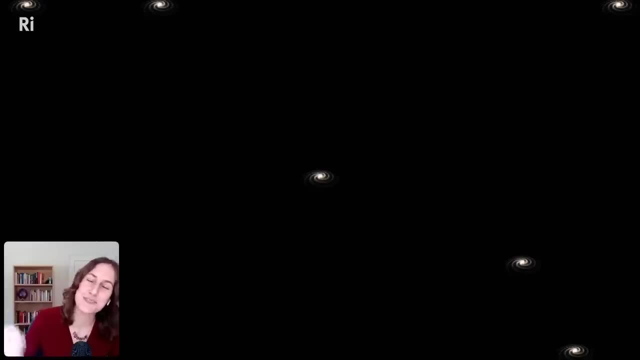 while looks like it's going to stop and then it just shoots off into space. It's really very similar physics. There's something strange happening in the cosmos that's making the universe expand faster. We don't know what that is. We call it dark energy. 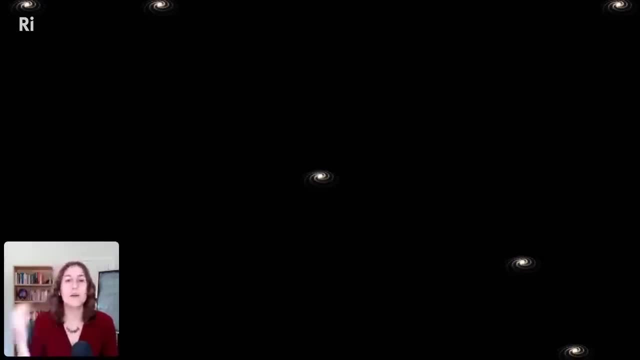 But it's something that's making the universe expand faster, And so, because of that, over time, each galaxy, or little clump of galaxies, if they're colliding with each other, is going to get more and more isolated. So our little group of galaxies, the local group of galaxies, we will collide with each. other. you know the Andromeda and Milky Way collision will happen. a little triangular galaxy will come in and get mixed up. But after that happens, in about 100 billion years, we will not be able to see other galaxies in the cosmos. We will not be able to see the distant galaxies. We won't be able to see the cosmic microwave background anymore. We will not know that there is anything beyond our little sphere of darkness, around our galaxy. The universe will become this increasingly empty place as things are moved away from. each other so far and so quickly that light can't travel between them anymore, And over time the stars in our own galaxy will start to die out and fade away. Matter will decay and even black holes will evaporate, and eventually we will be left. 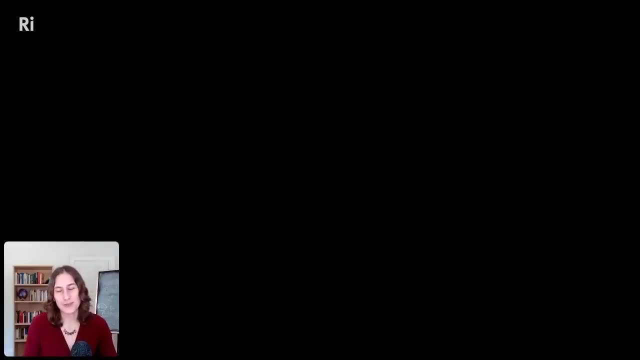 with a cold, dark, empty, lonely universe where all that's left is a tiny trace of the waste heat of all of the processes of the cosmos. That's called the heat death, And it's a very sad story. It's a rather depressing way to go, I think, if you're going to be a universe. 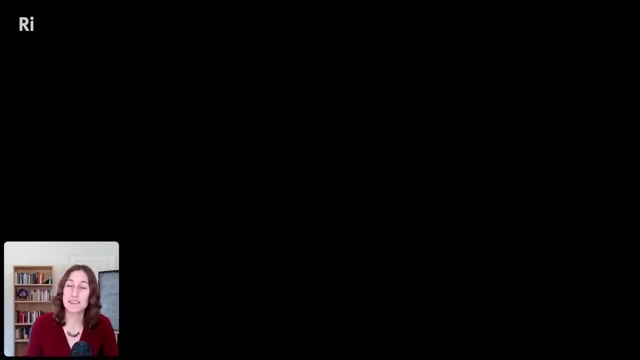 But it's also very gentle. It happens over a very long time. The time scale on this process is so long like you have to put exponents in the exponents to express how long this takes. So we're talking about 10 to the, 10 to the something years in the future. It's a very, very, very long time from now, But it happens slowly. it happens gradually and it's happening as we carry on. Already, star formation is slowing down. We have the peak of star formation, Something around I don't know- 10 billion, 9 billion years ago. And since then the stars have been forming less and less frequently. There have been fewer of these collisions of galaxies And right now you can calculate how many stars will be formed in the future versus how many have been formed in the past, And you can work out based on how galaxies are evolving and coming together. 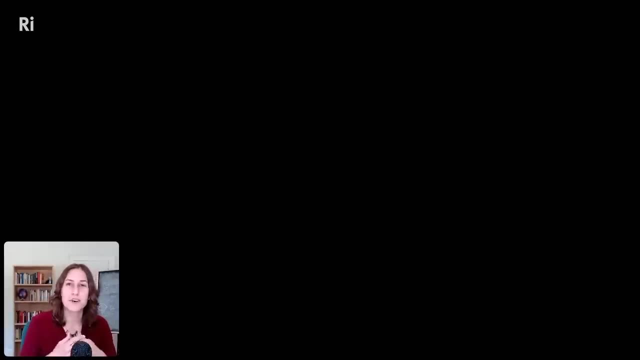 And you find that something like 90 or 95% of all of the stars that have been or ever will be have already been formed. So from now until the end of time, we're just working on those last 5%. It's kind of an arresting thought. 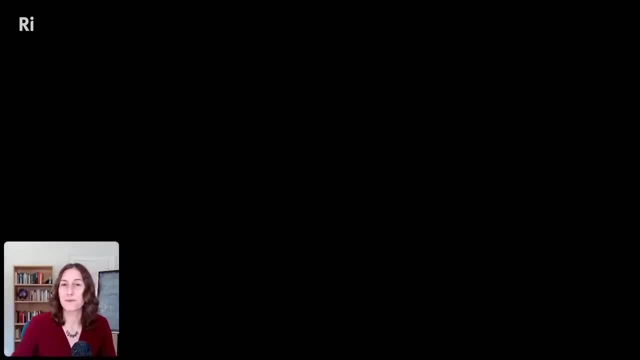 That from one perspective, the universe is almost done. From another perspective, we have so much time in the future, And so who knows what will happen. But that's just one possibility. There are still other ideas for how the universe might evolve, And a lot of the uncertainty comes from the fact that we don't understand dark energy. We don't understand what it is, the stuff is that is making the universe explode, And we don't understand that dark energy is exactly what it is that's making the universe explode, And we don't understand this energy And we tend to wonder: what does it mean for us? 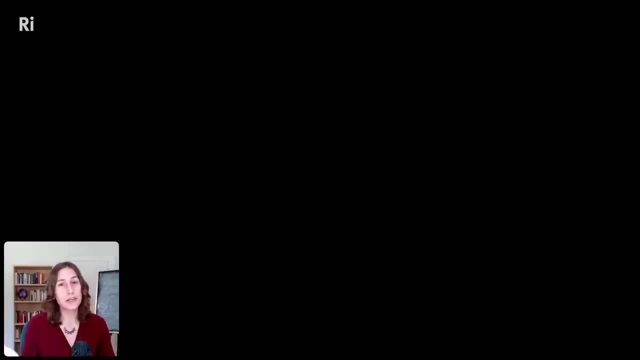 We tend to wonder what this energy, is, this universe, And we tend to wonder what does it mean for us. What does it mean for us is that it's making the universe expand faster And it could be weirder, which leads us. 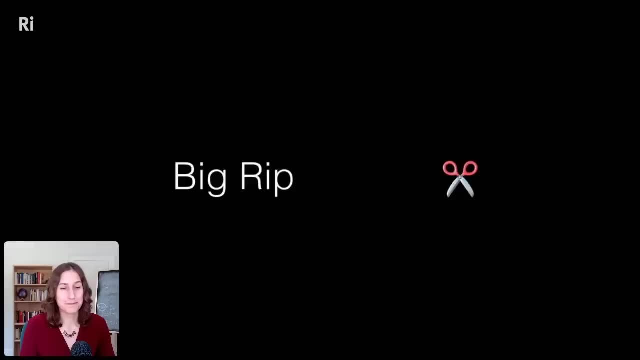 to the next scenario: the big rip. So the big rip is based on the idea that maybe dark energy is something stranger than what we generally assume it is. So the usual assumption about dark energy is that it's something called the cosmological constant. 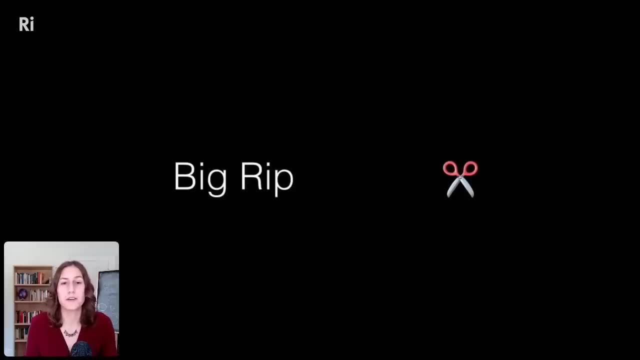 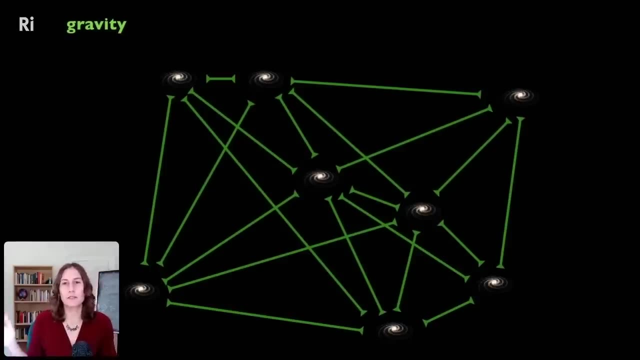 Cosmological constant is something that Einstein first came up with to solve a problem in cosmology. The problem was that the universe should have destroyed itself already. So if you look out into the universe, if you don't know that the universe is expanding. 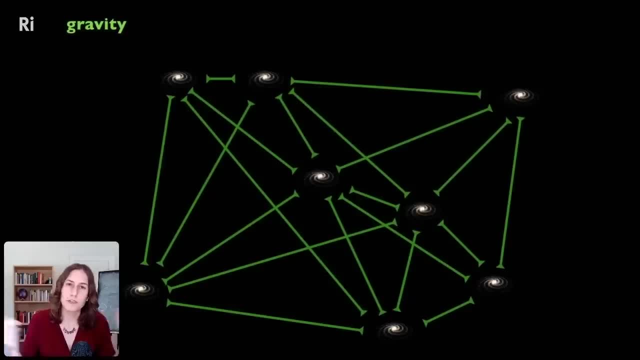 then you see there are galaxies out there And those galaxies should be pulling toward each other And they should just all come together and be one super galaxy. Their gravity should pull them together And when Einstein was first looking at this problem he didn't know the universe was expanding. He also didn't know there were galaxies outside of our galaxy. He was just looking at the stars and seeing that the stars were expanding. The galaxies weren't coming together. It works just as well with galaxies as the argument at the time did with stars. But he thought: how is this all staying out there? Why isn't the gravity pulling everything together and making it collapse? He didn't know that the Big Bang set off the expansion, So he had to put something into his equations to counteract the gravity of everything. 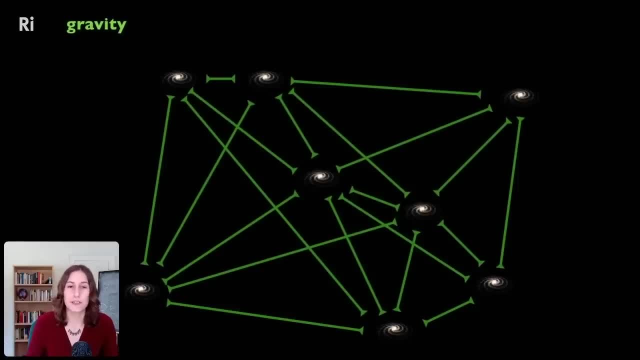 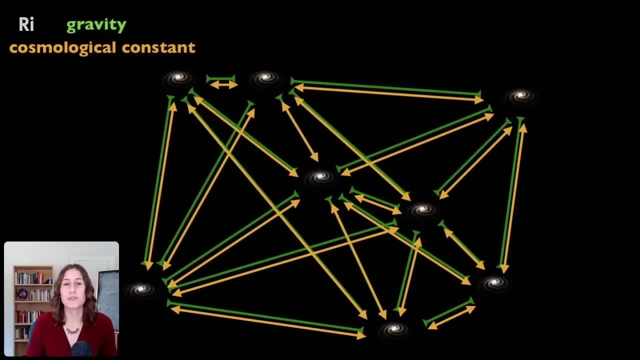 out there in the universe to keep it from falling in and just collapsing immediately or having already collapsed before. So he put in a term And in equations called the cosmological constant. And the cosmological constant was there to kind of balance the gravity of all the stuff. 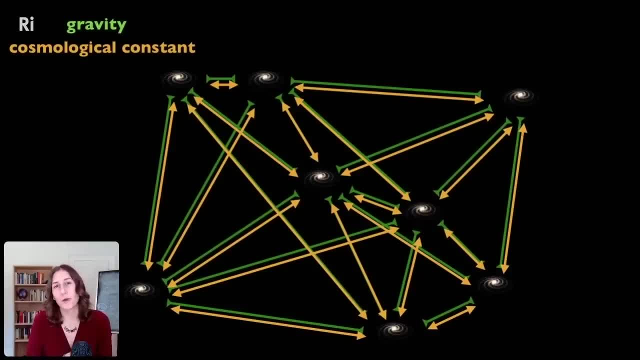 in the universe. So it was a property of space, a property of gravity, just something where every part of space has a little bit of stretchiness in it that kind of pushes against, just kind of expands the universe and exactly counteracts the gravity of everything. 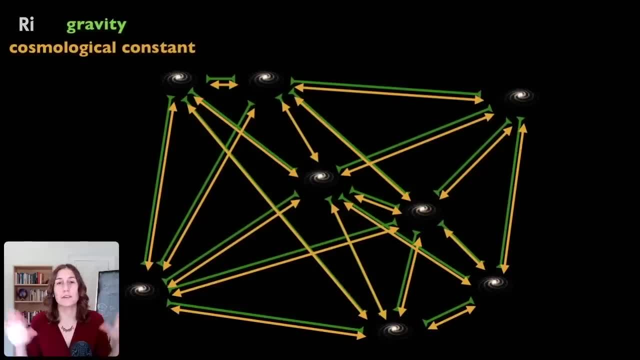 trying to pull the universe together And the idea was to keep the universe stable and steady When it turned out that the universe was still there, when it turned out that the universe was not steady, when it turned out that the universe is actually evolving. 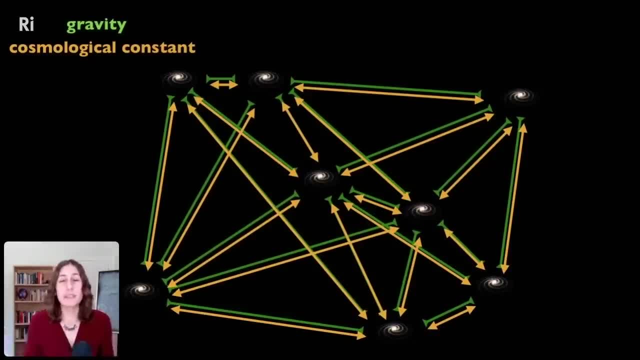 is expanding. he took the cosmological constant away because you don't need it anymore. If the universe is expanding, then it's just sort of like the momentum from that expansion that keeps the universe from having already collapsed. So there's the gravity that's slowing down the expansion. 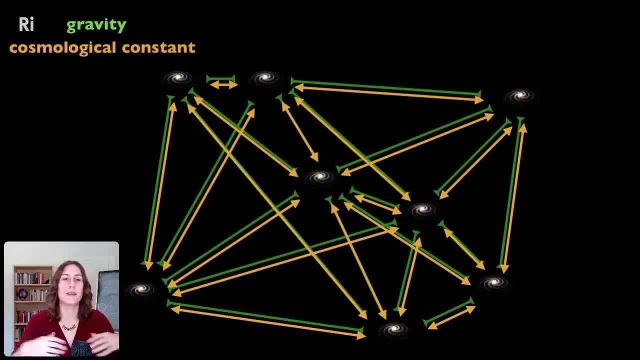 but it doesn't immediately make it stop. So the Big Bang set off this expansion. The gravity might be slowing it down, But you don't need a cosmological constant to keep the universe from having already been destroyed in the past. But then, when the universe was found, 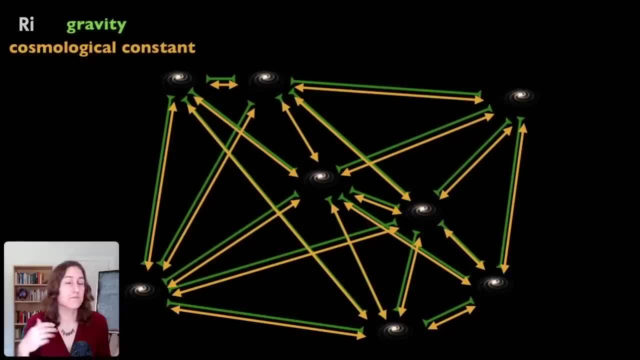 to be accelerating in its expansion. we needed something in the universe that could be pushing out, that could be stretching space, to keep the expansion going, even though there was gravity pulling everything in. And so we put the cosmological constant back in And we said, OK, maybe there is something. 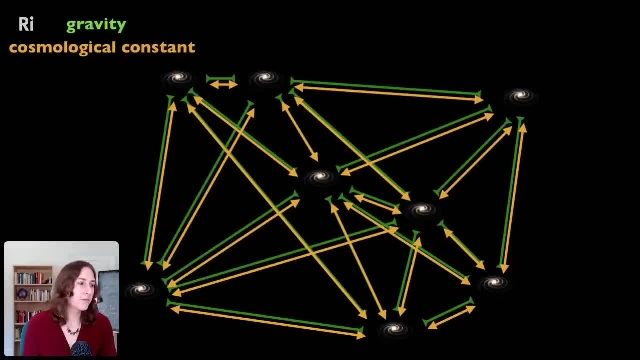 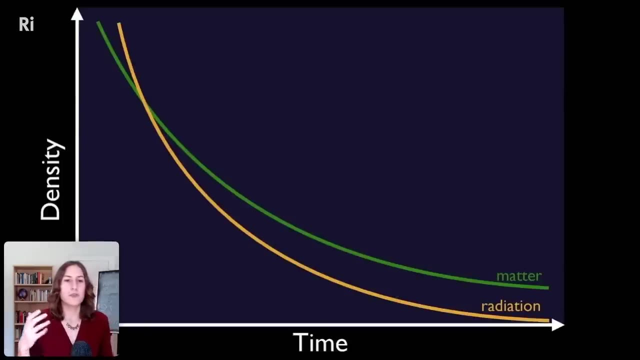 about every little part of space that makes it want to expand faster. If you do that, then you find that that leads to a universe that's just expanding, that has very little matter in it. that leads you to a heat death, Because basically, what it looks like is, if you look at the density of things in the universe, 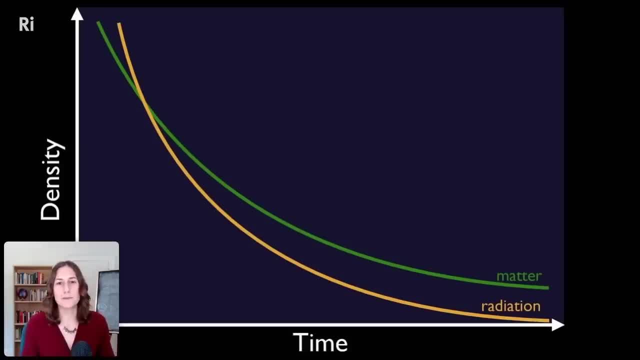 versus time. then over time, as the universe is expanding, the density of matter is dropping, because you have the same amount of matter but a larger space, And so the density of matter is dropping. the density of radiation is dropping even faster because, as the universe expands, not only does the amount of radiation inside the 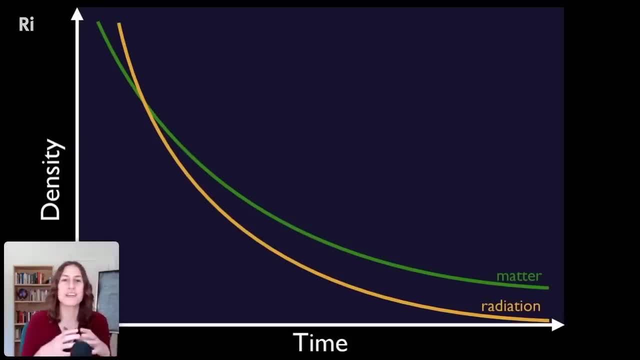 cosmos go down, but also it gets kind of stretched out to lower energies. So as the universe is expanding you're diffusing both matter and energy. But dark energy, if it's a cosmological constant, is just a property of space. 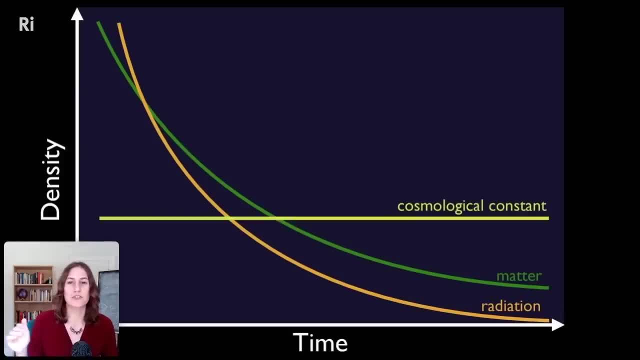 So when there's more space, there's more dark energy, And so the density of the cosmological constant is just totally the same, And that means that eventually you're going to have a situation Where the matter and radiation have been so diluted out that basically all that's left. 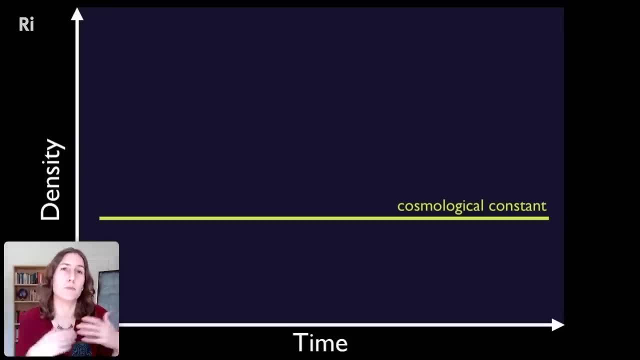 is cosmological constant. That's how you get to a heat death is you know, the universe is basically empty, other than this, whatever it is that's making the universe expand faster. But the heat death is gentle in the sense that a cosmological constant can move galaxies. 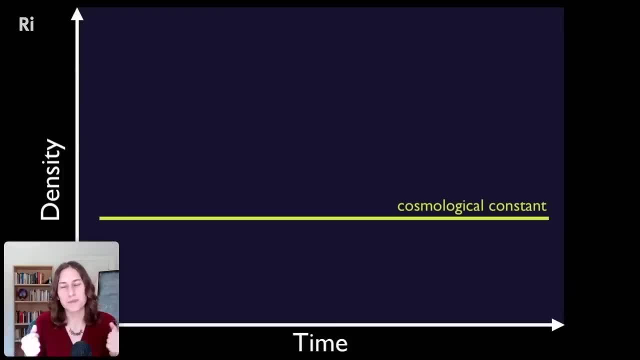 apart from each other, but it can't rip galaxies apart themselves. Like the amount of dark energy, the amount of cosmological constant in a volume doesn't increase over time. So you don't You don't get things that are already sort of orbiting each other being pulled apart. from the expansion of space within them, because it just doesn't work that way. But there could be a different kind of dark energy that's not a cosmological constant where the density of it actually increases over time, Where within a galaxy you could get more and more dark energy, kind of popping up in that. 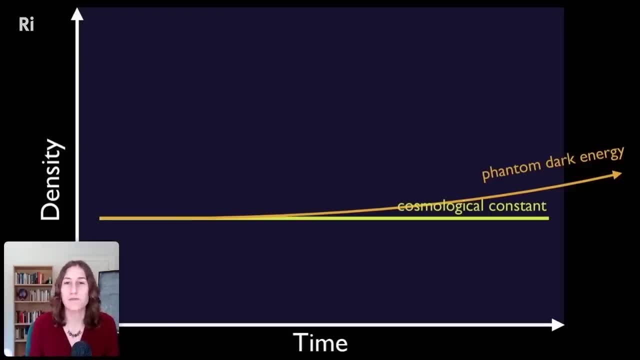 space and stretching apart the galaxy, And that's called phantom dark energy. It's a hypothetical possibility for how dark energy could work. It's not. It's not the most accepted idea. There are sort of theoretical reasons to think that maybe it doesn't fit with our understanding. 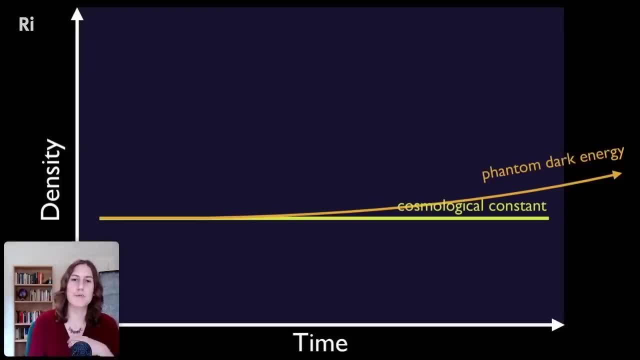 of how energy works in the universe in quite that way. But if it were true, then it would lead to a total destruction of the cosmos, because not only would galaxies be moved apart from each other, they would also be torn apart themselves. And if dark energy is increasing in every point in the universe over time, then you 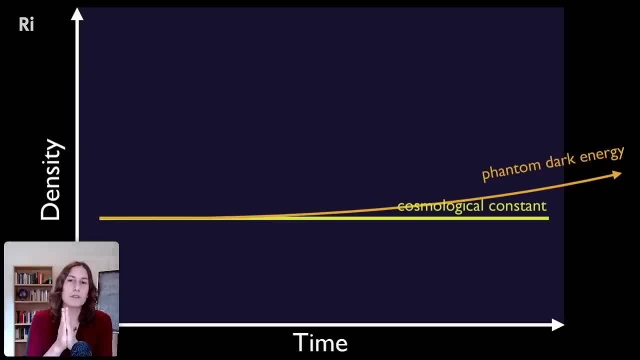 get to a stage where, no matter how close together two things are, The expansion of the universe is so violent that it moves them out to infinite distance, Which means that you're ripping apart fabric of space itself, And that leads to what we call the big rip. 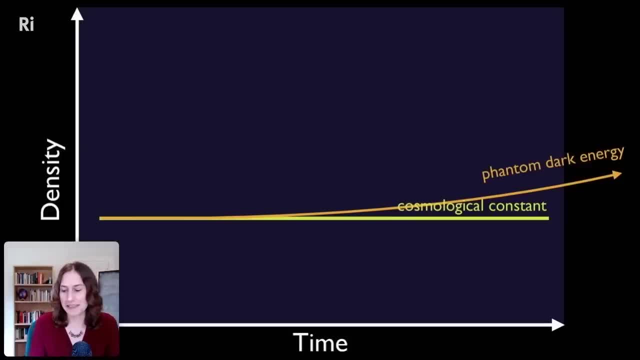 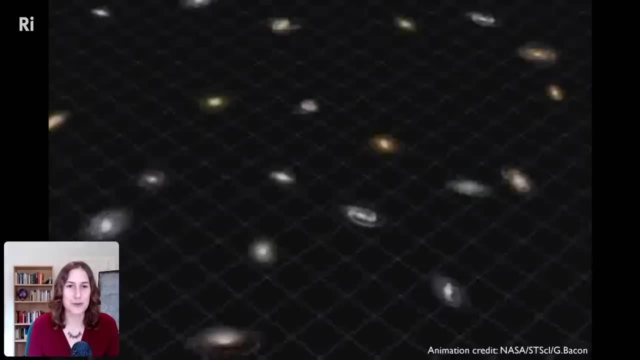 So a few years ago there was a paper about this And NASA made an animation to describe what the big rip would look like if it happened. And I'm including this animation because I think it's, I think it's just such a cool. 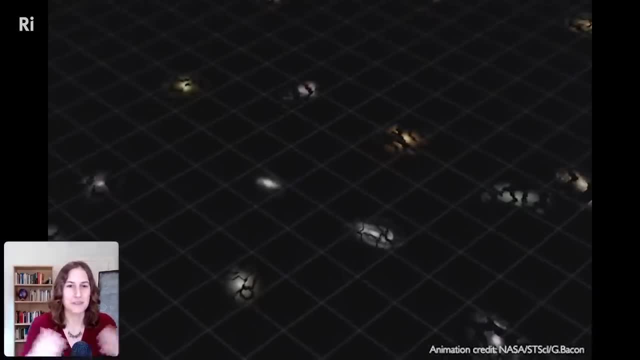 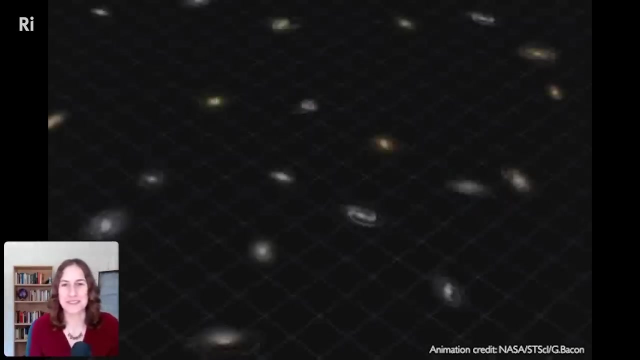 Such a cool diagram. So you have the expansion. then, oh no, the galaxies get torn apart. So let that play a couple times: Universe expands, galaxies get farther apart, and then they're disintegrated and the whole universe is destroyed. 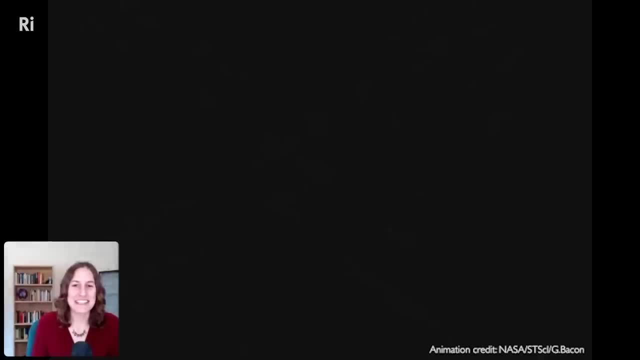 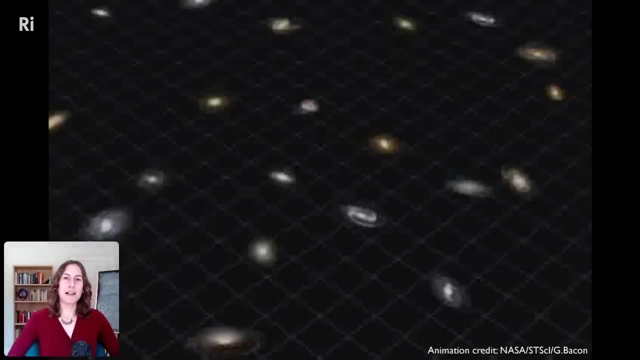 I think that's a. I think that's kind of a neat possibility for an end of the universe. It's a very violent one, So okay, So do we have to worry about a big rip? Is this something that's going to happen to us? 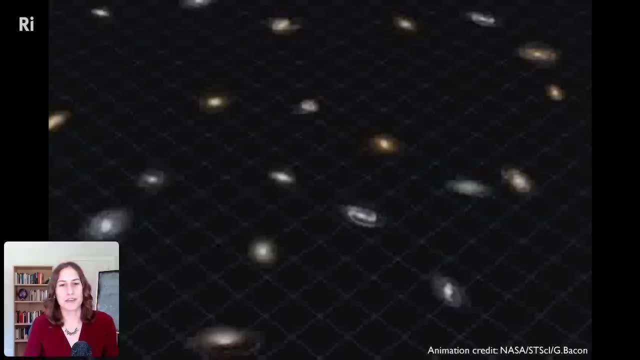 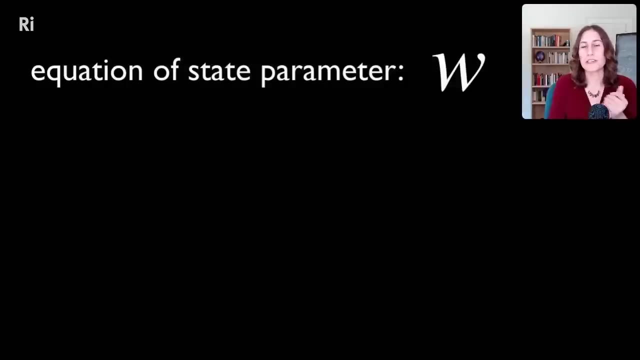 Well, in order to know if a big rip is coming, we have to know something about dark energy, And what we specifically have to know about dark energy is something called the equation of state parameter. This is written as W. It's a ratio of the density and the pressure of whatever. this. 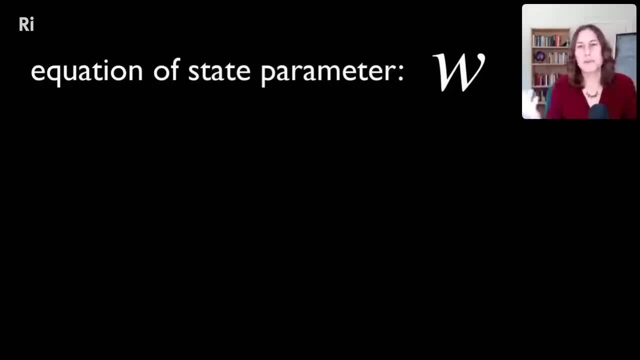 stuff is that's making the universe expand, expand faster. The only thing you really need to know about the equation of state parameter right now is that, If it's a logical constant, the number is exactly negative one, And so we can do various ways. 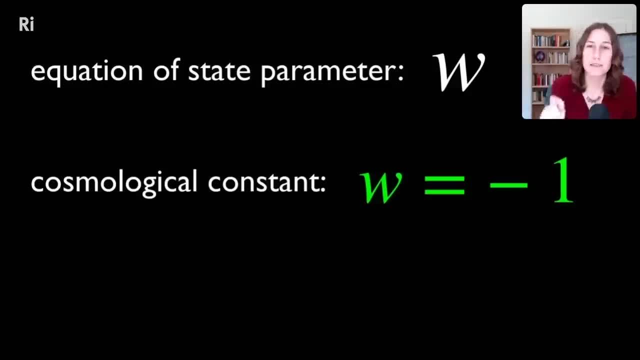 We can measure the equation of state parameter to see if it is exactly negative one. If W is anything less than minus one, any little bit less than minus one, then you get a kind of dark energy that increases in density over time and that will eventually destroy. 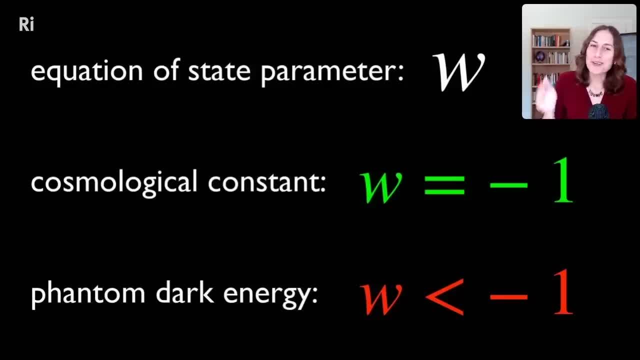 the universe. So if W is less than minus one, then you can calculate exactly- Okay, Exactly- how long in the future the universe will be destroyed. You can work out when all sorts of various things will be destroyed. You can get a date for the big rip. 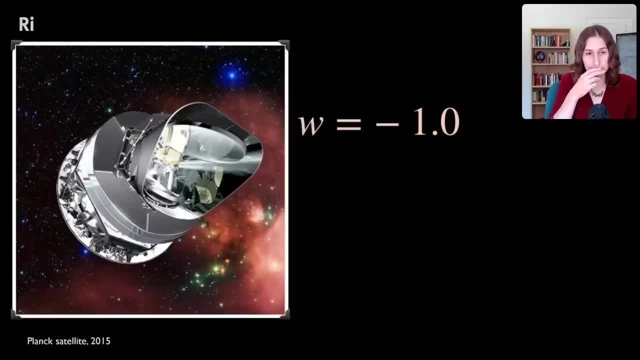 Okay, So what have we measured for W? Well, this is the Planck satellite. It's the one that gave us that picture of the early universe, the cosmic microwave background, And it can measure. It can measure W, It can determine what W would be. 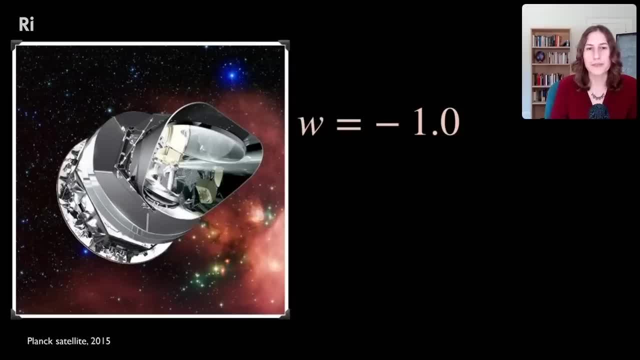 And it gets a number that's, you know, to a first approximation minus one. But if you actually write down the whole number that's been measured, you get negative 1.028 plus or minus 0.032.. What that means is that the idea that W is exactly minus one is still included within. 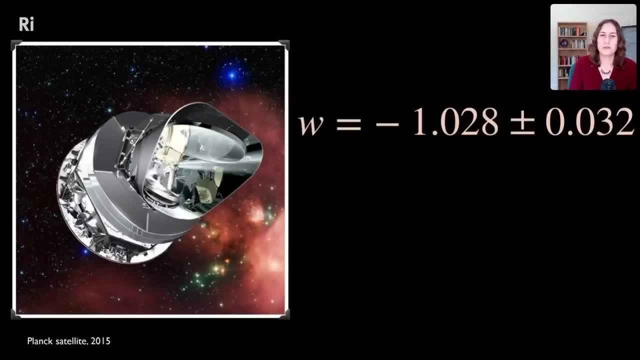 the uncertainty of the measurement. We could be off by 0.032 on this, On this number that we've measured, But it also means that the value could very well be less than minus one And if we work out the sort of earliest that the 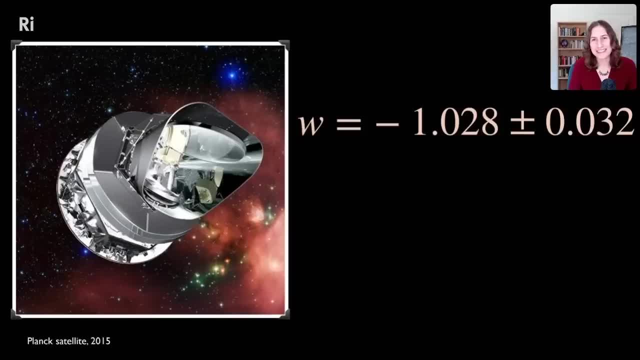 The earliest that the cosmic doomsday could happen based on this measurement, based on the uncertainties within this measurement, then the soonest it could possibly happen is about 188 billion years from now, Which means we have at least about 188 billion years before the universe tears itself apart. 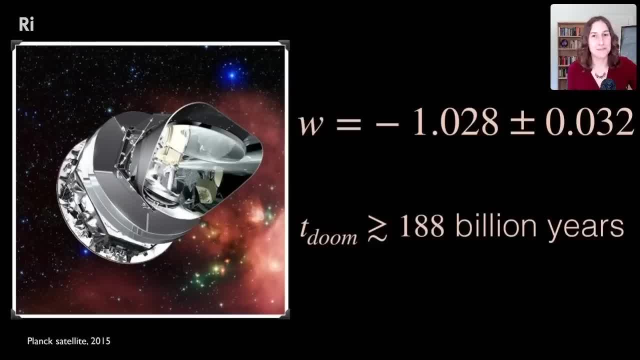 Okay, So probably it's never going to do it at all. Probably we'll just keep measuring that number and get more and more accuracy and push that cosmic doomsday farther and farther into the future. But we'll never be able to measure W to such perfect precision that we can completely rule. 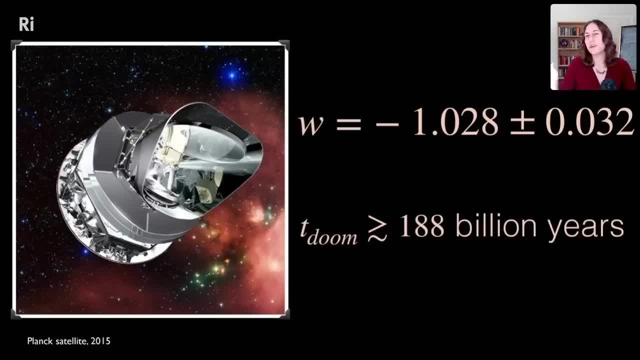 out the idea that we could have this phantom dark energy. Maybe we'll find some theoretical reasons why it really can't happen. But in terms of the data at the moment it slightly prefers something that looks more like phantom dark energy than not. But again, as I said, if you talk to theorists they'll say, oh, this is not a good idea usually. 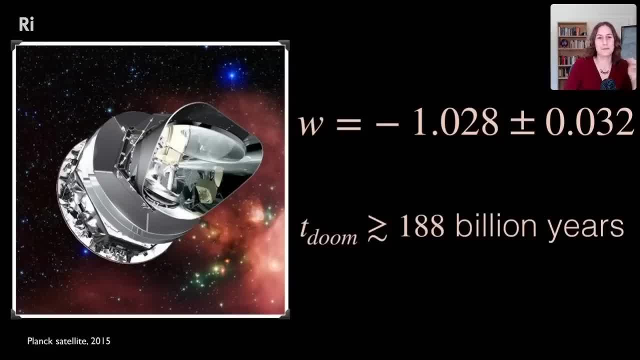 But you know, it's something that's a possibility. We can't rule it out with the data, So we have to- you know, might as well think about what it would look like. So you know, that's 188 billion years, plenty of time. 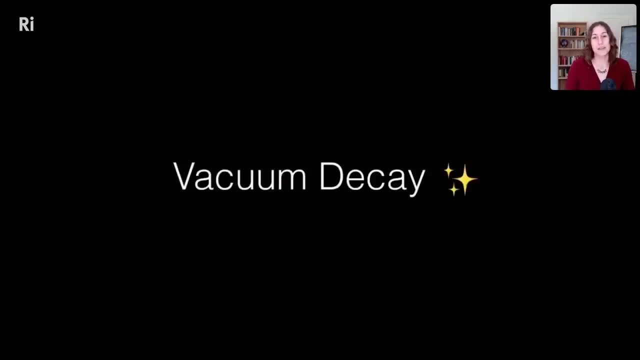 There is one possibility for the end of the universe that technically could happen at any moment. I am going to put a disclaimer here right now to say: do not worry about vacuum decay, and I'll come back to why you should not worry about vacuum decay destroying the universe. 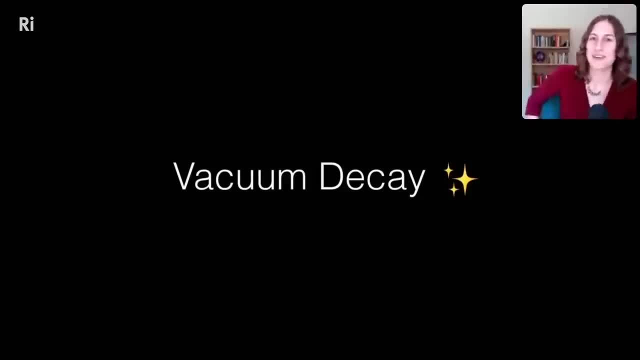 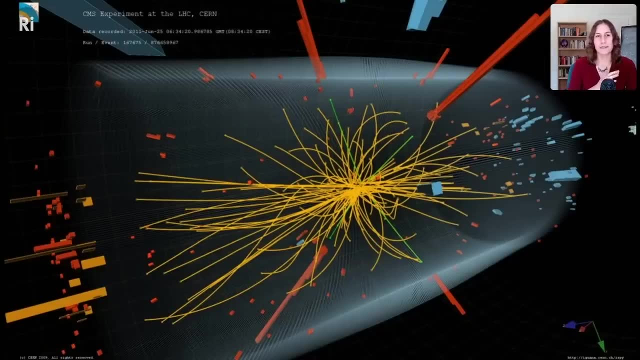 at any moment, But for now, let's just talk about the physics of what that means. So in 2012, there was a discovery at the CERN facility at the Large Hadron Collider, where they smashed protons together and they found evidence for a particle called the Higgs boson. 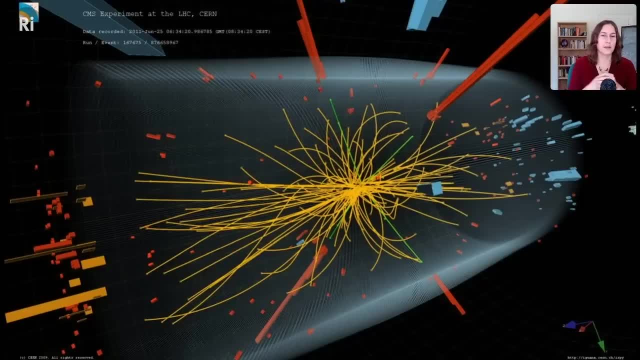 Now the Higgs boson is a particle associated with what we call the Higgs boson. It's a particle that's called the Higgs boson. The Higgs field is an energy field that pervades all of space and has something to do with. 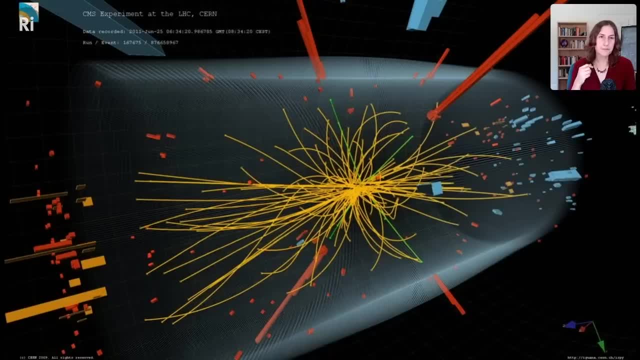 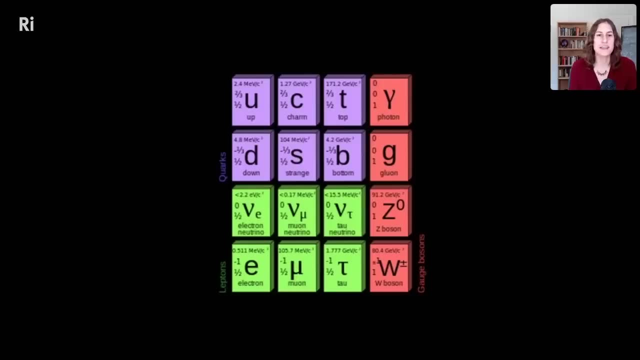 how particles got mass in the early universe And when the Higgs particle was discovered. it kind of completes the standard model of particle physics. So the standard model of particle physics is this collection of all the particles we know about in the universe from all the experiments we've ever done in laboratories. 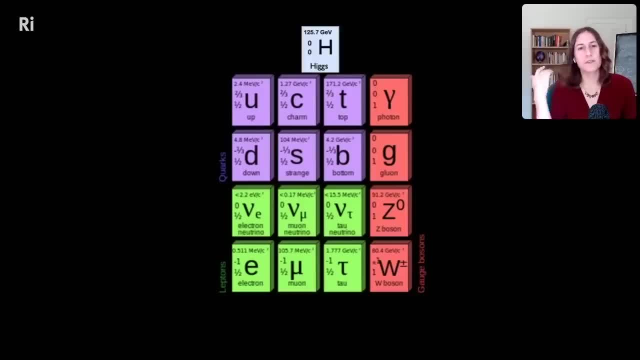 So there's this set of particles that we had already discovered, And then there's the Higgs boson, which kind of is part of this picture now as well. So I'll just walk you briefly through what these particles are: The blue, purpley ones, those are the quarks, which are the most famous of these are the. 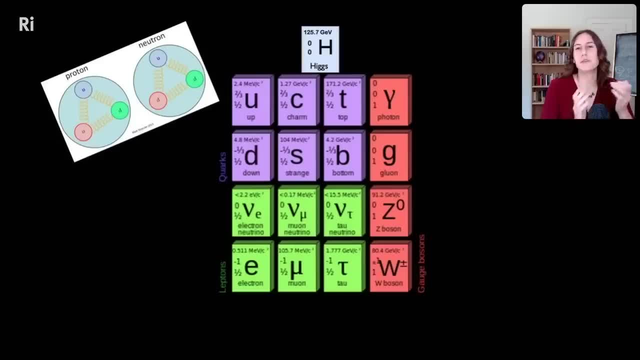 up and down quark, because the up and down quark are components of the proton and the neutron, these particles that live at the centers of atoms. Then the green particles there, those are the leptons. So the most famous lepton is the electron, which is the one that orbits the centers of 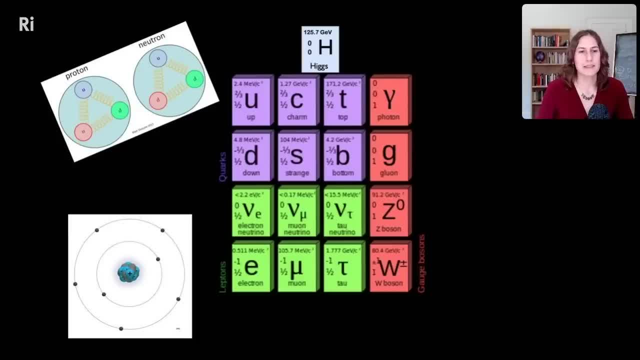 atoms. Or if you think about it in a quantum mechanical sense, it exists sort of in this cloud of probability of electron-ness surrounding the center of an atom. But there's the electrons and the electrons particles, the muon and tau, the sort of cousins. 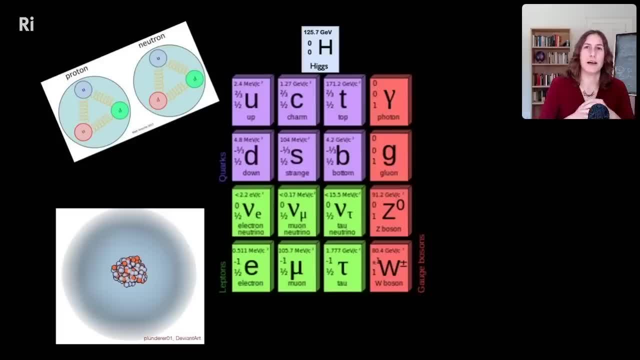 of the electron. And then there's the neutrinos which are produced in nuclear fusion and among other things, And those just kind of pass through the earth all the time. They're these sort of ghostly particles. Then on the right there's the gauge bosons. 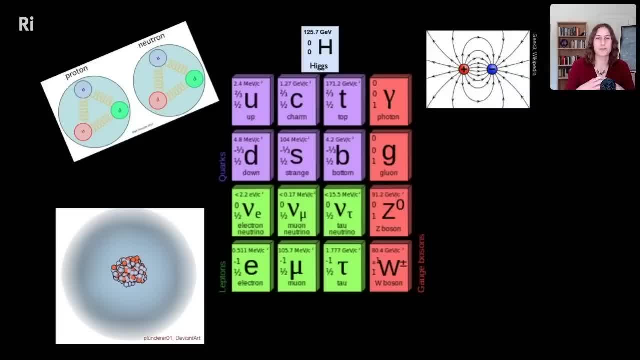 These are the red ones. These are the force carriers, So the particles responsible for the forces of nature. There's the photon, which is responsible for electromagnetism. So light is made of photons and electromagnetism. magnetic fields, electric fields, those are. 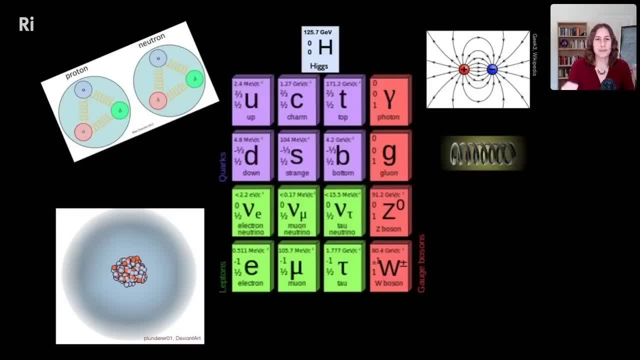 all mediated by photons. There's the gluon. This is the mediator of the strong nuclear force. That's what holds protons and neutrons and quarks together in the centers of atoms. And then there's the W and the Z bosons, which mediate the weak nuclear force. 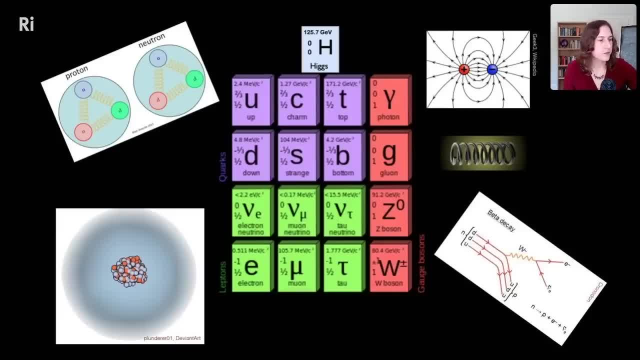 Those are responsible for things. They're responsible for things like radioactive decay, And by measuring the properties of all these particles we can get an idea of the stability of particle physics. We can get an idea of how well the standard model of particle physics works, in the sense. 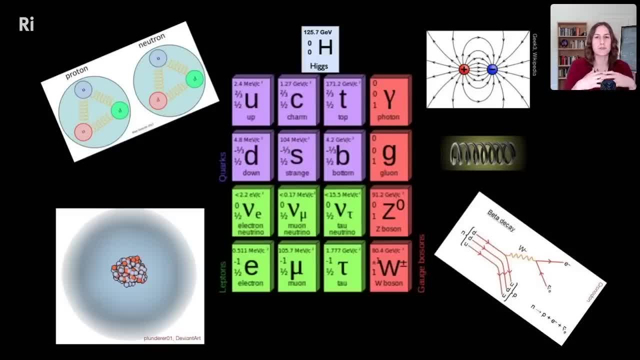 of whether or not this is the sort of optimal arrangement of particles and fields for a universe like ours. So, to make it a little bit easier, I'm going to stop here. I'm going to make it a little more concrete. The Higgs field, this energy field that pervades all of space, has a value to it. 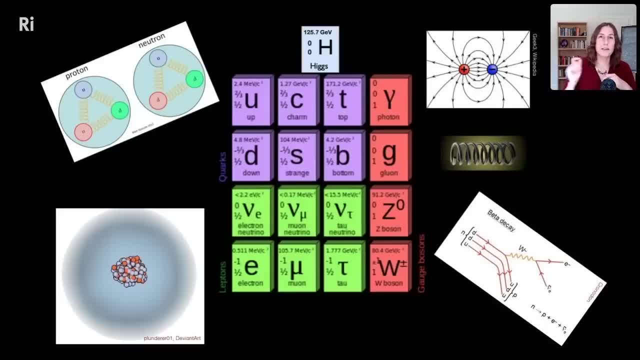 So there's this sort of number associated with the Higgs field, And the value of the Higgs field determines it's tied into the forces of nature, the constants of nature, how particle physics works. And in the very early universe the Higgs field had a different value than it does today. 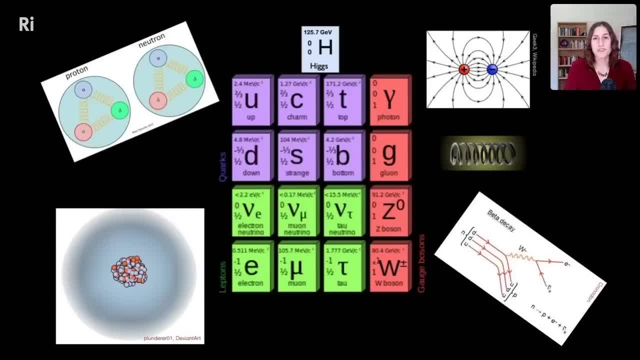 And in that time we had a different mix of particles, A different mix of like particles, Like forces of nature, And atoms and molecules didn't exist in the way that they do now. When the Higgs field switched, it changed its value. 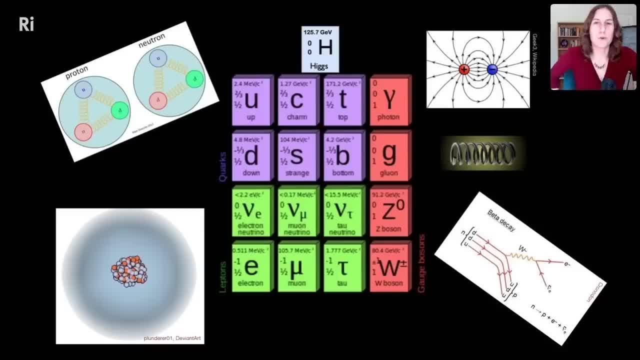 That allowed certain particles to get mass. We are able to have protons, electrons and neutrons and everything And particles you know, atoms and molecules can hold together and we can have structure and stars and planets and people and everything is great. 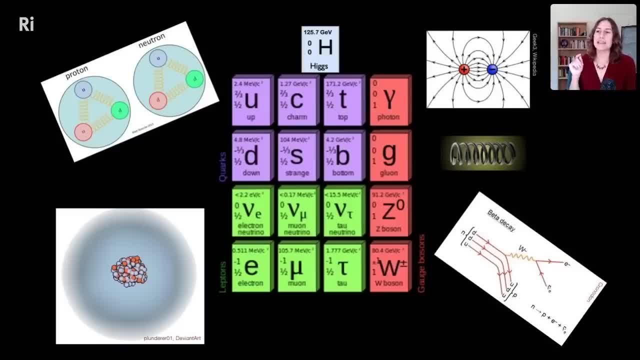 So we like having the Higgs field at the value it is, And the problem is: there's a change. There's a change, There's a chance that the Higgs field could prefer in some sense, a different value. It could be vulnerable to changing again. 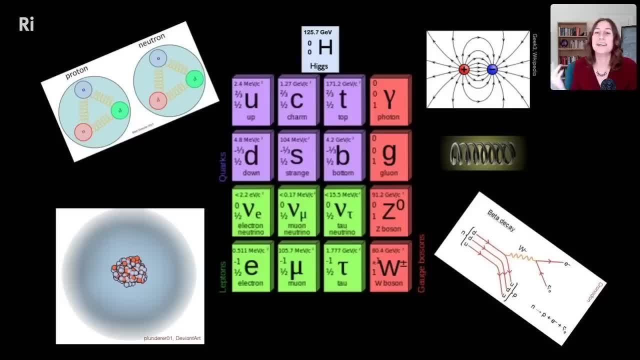 We don't want that to happen because we want our particles to stay together, But there's a chance that it's vulnerable to changing again, that it's not fully stable. So we can use the measurements we've done around the Higgs, boson and other particles. 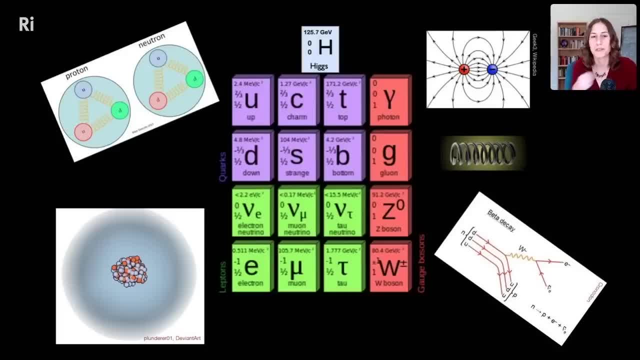 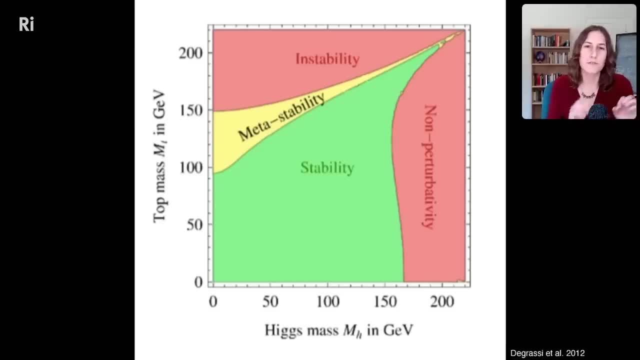 from the standard model of particle physics. specifically, the top quarkus is one that's used for this measurement, And we can plot out different regions. We can look at different possible combinations of values of the masses of these particles, where you get a universe that is stable, where the Higgs field just wants to stay where it's. 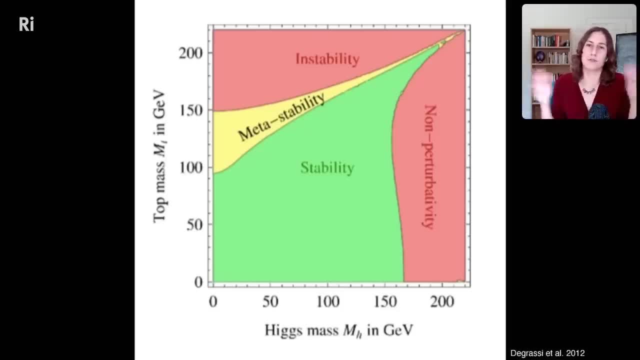 at or a universe that's not stable, or one where the sort of math doesn't even work out. So in this diagram imagine that the Higgs field, the Higgs particle, excuse me, has a mass of 50 GV. So GV is a measurement of energy or mass for these kinds of particles. 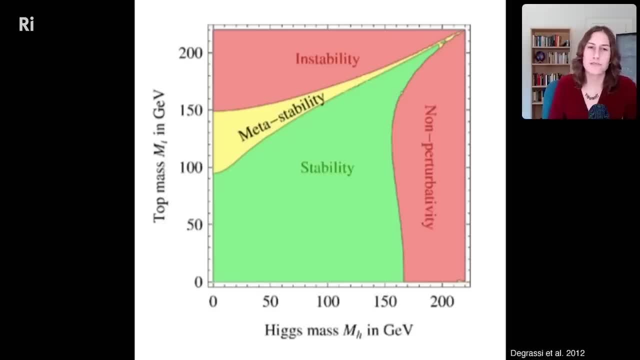 So let's say the Higgs particle has a mass of 50 GV. So GV is a measurement of energy or mass for these kinds of particles. So let's say the Higgs particle has a mass of 50 GV. So the Higgs particle has a mass of 50 GV. top particle has a mass of 50 GV. 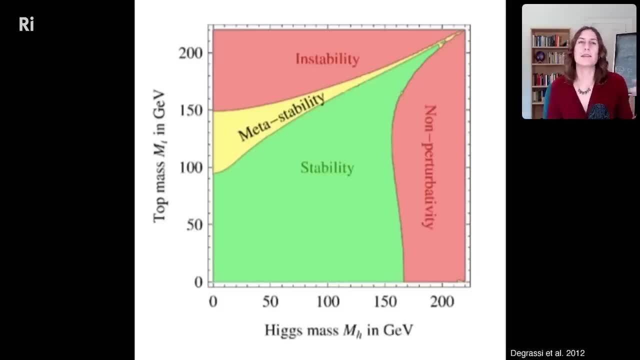 Then we're squarely in the stable part of this diagram. Then that would mean that the that the the Higgs field wants to stay at the value it's at forever and everything's great If the Higgs field, if the Higgs particle had a mass of 50 GV and the top mass was 200,. 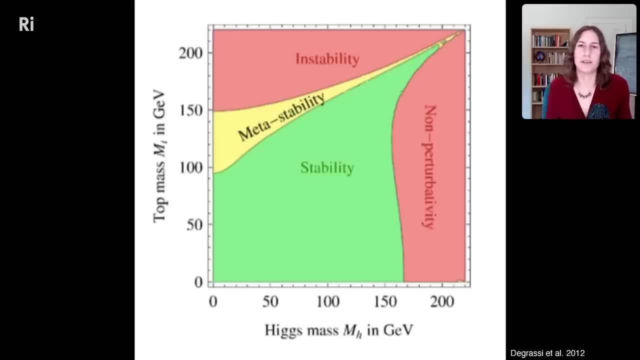 then we'd be an unstable universe, have already destroyed itself. you know That we clearly don't live there. So if you actually put in the masses of the particles is measured, you find we live right there, Right in that little slice of meta-stability which means that the universe is stable now. It means that the Higgs field. 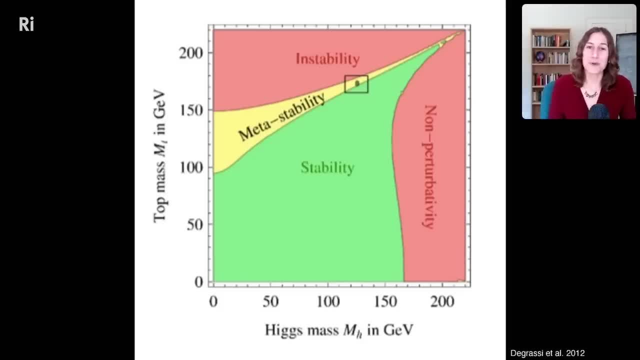 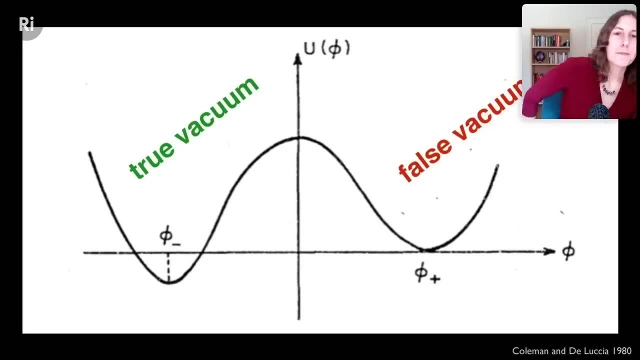 is not immediately changing but is very vulnerable to change in the future. So to give, to make this a little more concrete, imagine that. so this is a sort of diagram of two possibilities for the Higgs field. So each little valley in this picture you can imagine as you can. 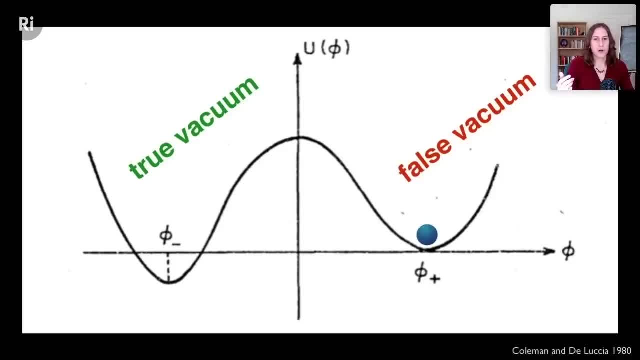 imagine like an actual valley with, like you know, maybe there's a little ball sitting in the valley And the lower one is the true vacuum. That means it's the. it's the valley that the Higgs field would rather be in. Imagine that little ball is the Higgs field And there 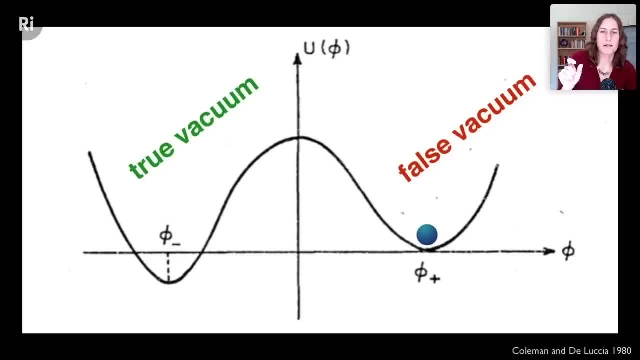 are these two little valleys And there's the false vacuum which is like where it's sort of stable. It can hang out in that little, that little valley, But if you gave it enough of a kick it would fall into the true vacuum. It would. 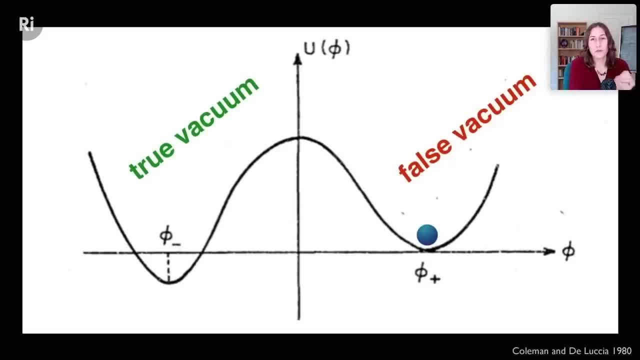 fall into that, that true vacuum valley, And that would be where it was most stable, Where it would it would you know, stay forever. So you can think of, you know, something that would disturb the Higgs field, make it go over that bump, end up in the true vacuum. 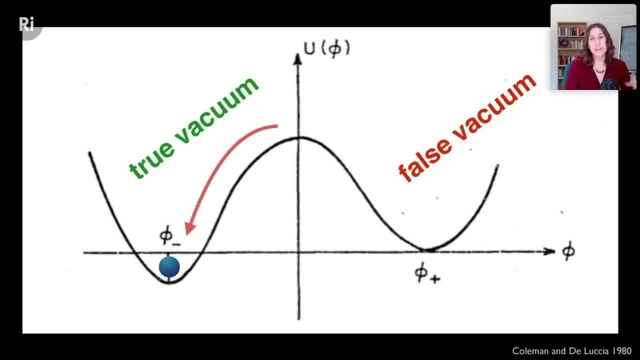 And that would be bad. right, Because that would be a different value for the Higgs field, And with a different value for the Higgs field, the constants in nature would be different, Our particles wouldn't hold together, And so you can imagine that the Higgs field would be. 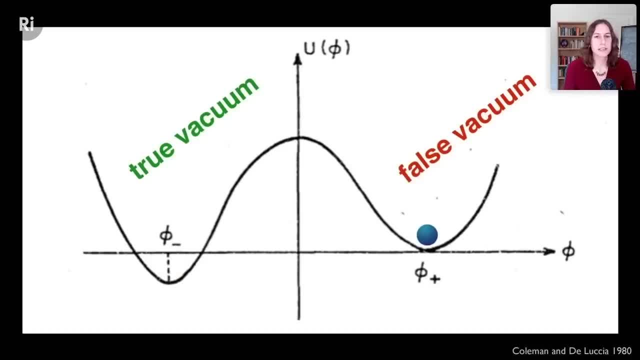 a disaster, right. So fortunately we don't know of any way to kick the Higgs field over that bump. There's no process of nature that we know of that could get to those kinds of energies. Certainly, certainly things like particle colliders can't disturb the Higgs. 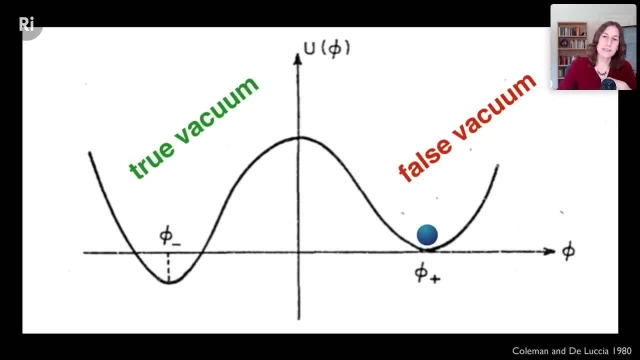 field that much. We know that because there are much higher energy events that happen in the cosmos And those haven't done it So and those have been happening for billions of years. So the idea that you know us sort of 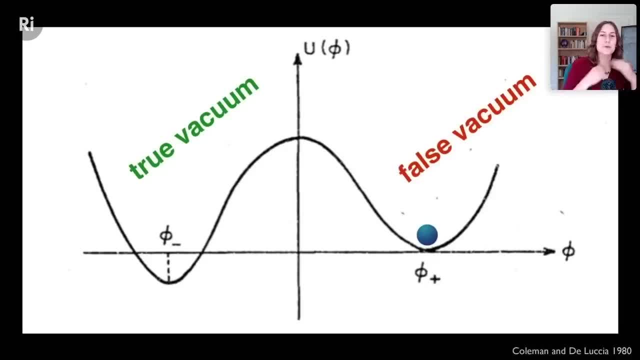 banging protons together could do. it is completely impossible. So we know that just a high energy event is not going to be able to do this. But the universe is fundamentally quantum mechanical, Which means that barriers are not always the barriers you think they are. 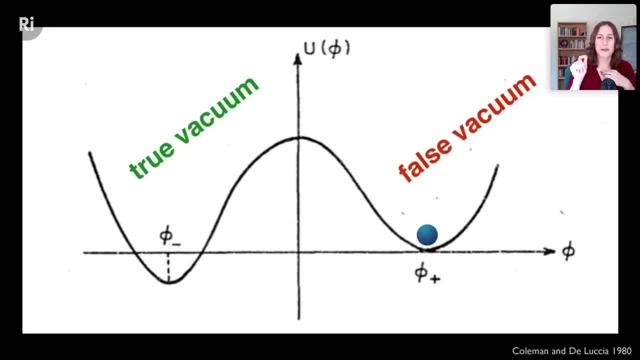 So whenever you have a particle on one side of a barrier in a quantum mechanical universe, there's a possibility that that particle could just show up on the other side of the barrier spontaneously through a process we call quantum tunneling, And this is something that has. happens all the time in electronics. We see electrons passing through barriers, tunneling through barriers in electronics all the time. We use it in certain kinds of microscopes, scanning tunneling electron microscopes. The whole point of them is to sort of leak electrons. 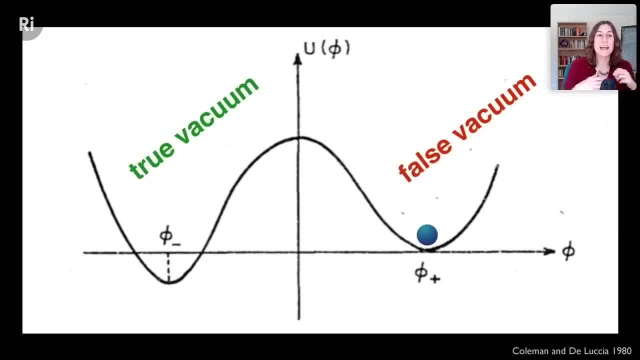 out through this quantum tunneling process, And it's the sort of thing that is not predictable, in the sense that you don't know exactly when a tunneling event will happen, but you can get an idea of the probabilities, of how long it will take, how long you'll have to wait. 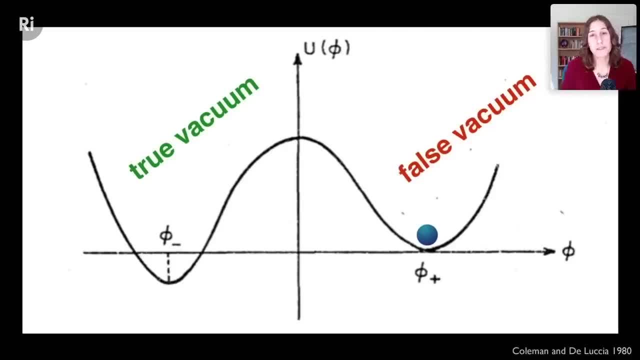 on average for this tunneling event to happen. But anyway, that kind of tunneling can apply to the Higgs field as well. So you can have the Higgs field sitting very nicely in its false vacuum state and if you wait long enough, eventually it will quantum tunnel straight. 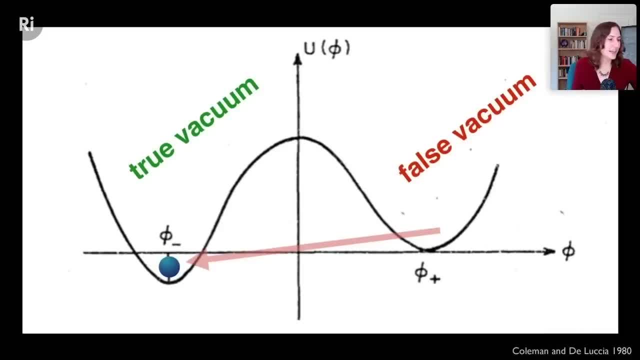 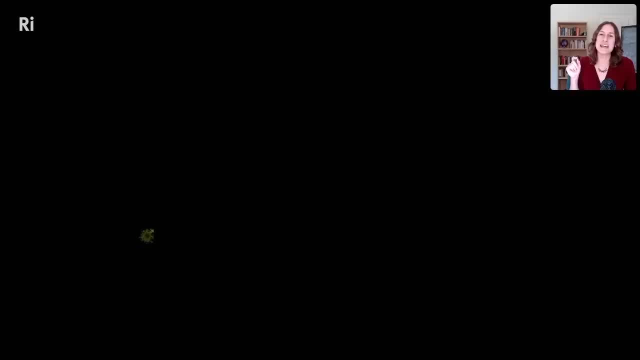 into the true vacuum, And if that happens, that's bad. So the way it would look is somewhere in the cosmos. So the way it would look is somewhere in the cosmos. So the way it would look is somewhere in the cosmos. You would have this quantum tunneling. 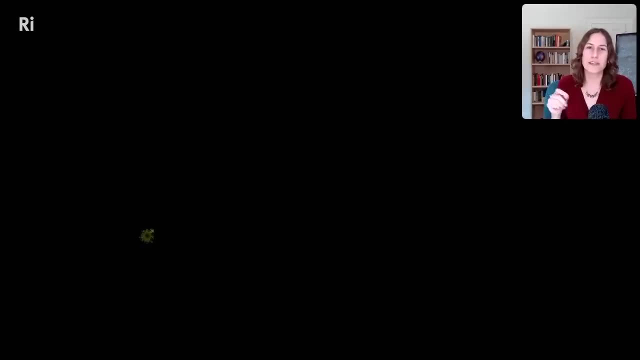 event happening at one point in the cosmos And that quantum tunneling event would produce, would change the Higgs field at that point, And then, through a cascade, it would change the value of the Higgs field and all the points around that point, And so you would end up. 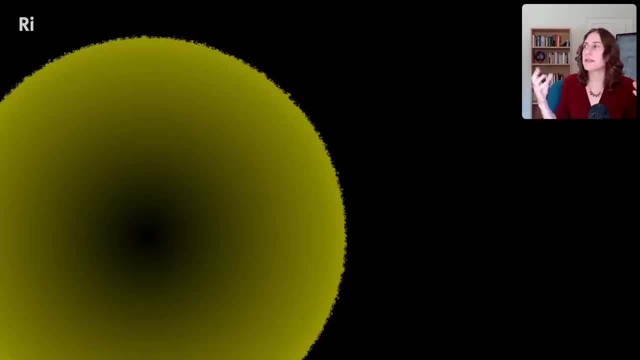 with a bubble of this true vacuum state, a different state of physics, a different arrangement of physics, where you have different constants of nature, where the particles don't hold together anymore, where you can't have atoms or molecules. You have a true vacuum state. 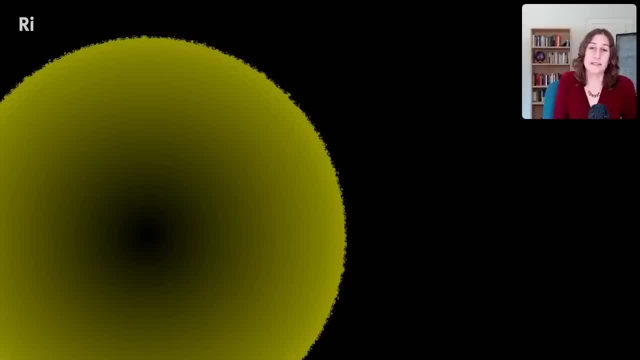 and a vacuum state of physics inside that bubble And that bubble has a bubble wall around it, a high energy shell of energy around that bubble And that bubble wall, as it goes through the universe, would incinerate anything it touches. That bubble expands at about the 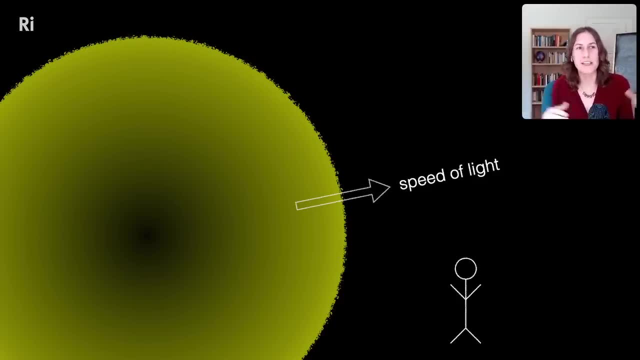 speed of light And because it's going at about the speed of light. if you're standing nearby, there's just no way you're going to see it coming, Because something that travels at the speed of light is invisible. Because, by the time, 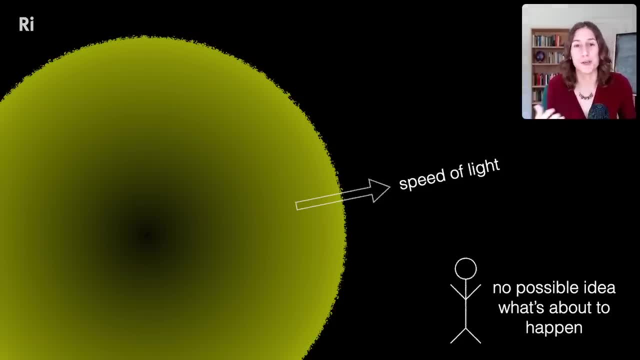 the light from it gets to you, it's already on top of you. There's no way to know that it's approaching. So I've told you that there's this possibility of this random event that could happen somewhere in the universe. We couldn't predict exactly when it would happen. 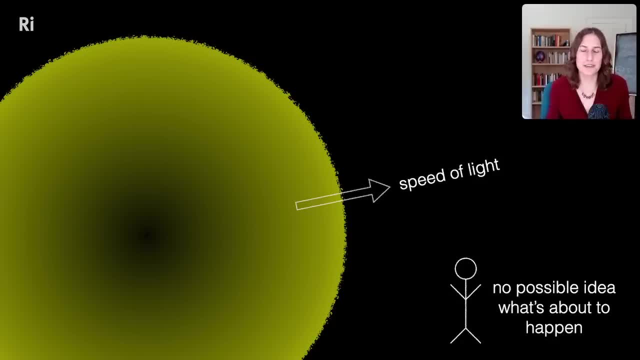 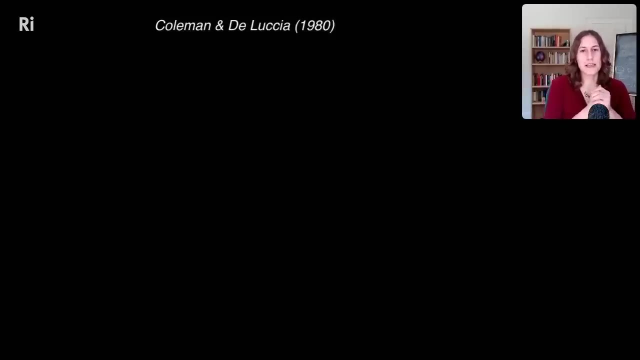 If it happened, it would create a bubble that expands at about the speed of light, destroys everything in its path. Now, when this was first discovered, there was this famous paper by Coleman and DeLucia in 1980, where they were talking about this. 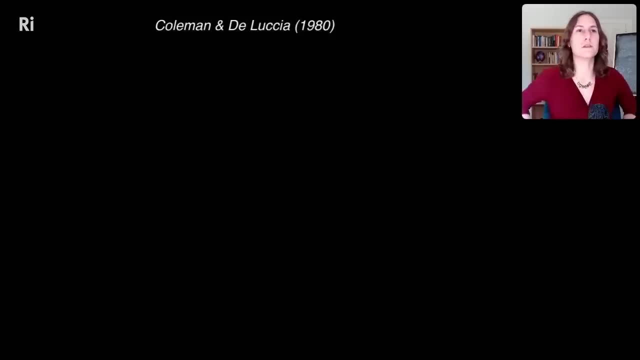 possibility. And they calculated not only- you know, they were not only just talking about what would happen if the bubble occurred, but they also calculated that the space inside the bubble, that true vacuum space, would be gravitationally unstable, Which means that as soon as something is inside the bubble, not only was it incinerated, coming in and then dissociated once it was inside the bubble, but the space inside the bubble was also going to collapse once it's there, because the particles can't hold together anymore. 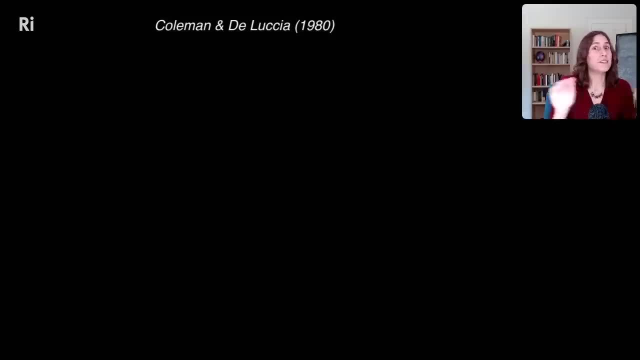 also. it would then collapse basically into a black hole. So it was real, real total destruction. And so in this paper they do this calculation and then they have a little discussion after the calculation. that is my favorite bit of physics poetry that I've ever seen in an academic. 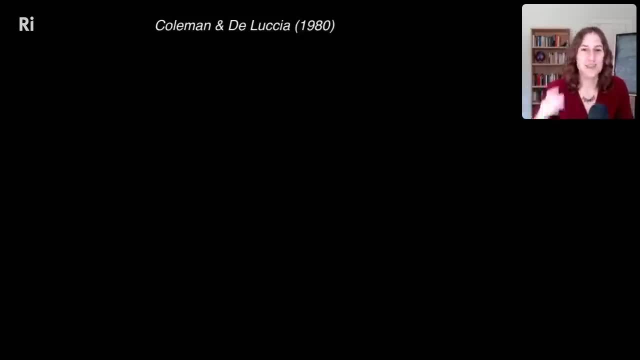 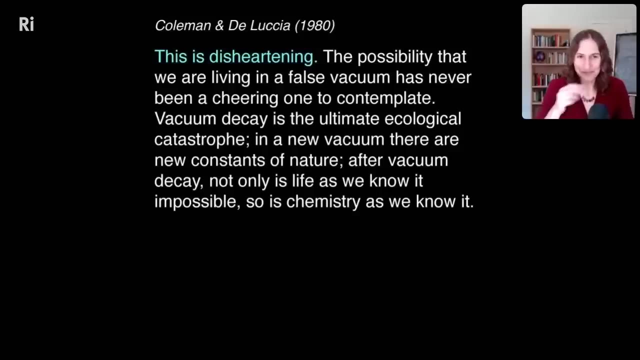 paper. So I'm just going to read you a little piece of that discussion. So they just calculated that the false vacuum is going to collapse or the true vacuum is going to collapse on itself. So they say: this is disheartening. 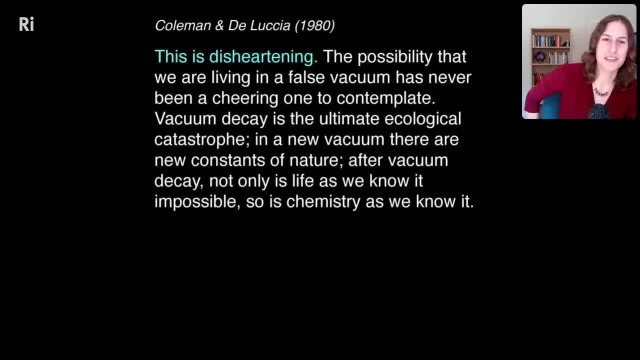 The possibility that we are living in a false vacuum has never been a cheering one to contemplate. Vacuum decay is the ultimate ecological catastrophe In a new vacuum. new constants of nature. after vacuum decay, not only is life as we know it possible, so is chemistry as we know. 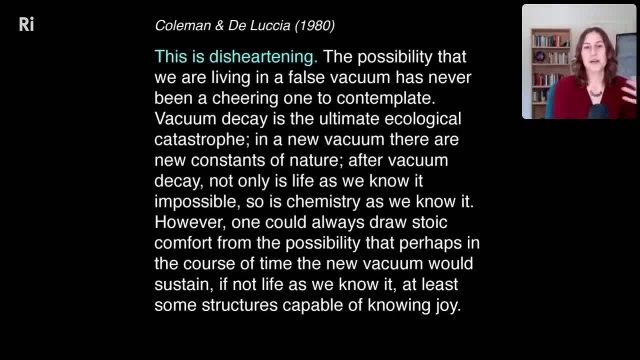 it. However, one could always draw stoic comfort from the possibility that perhaps, in the course of time, the new vacuum will sustain, if not life as we know it, at least some structures capable of knowing joy. This possibility has now been eliminated. 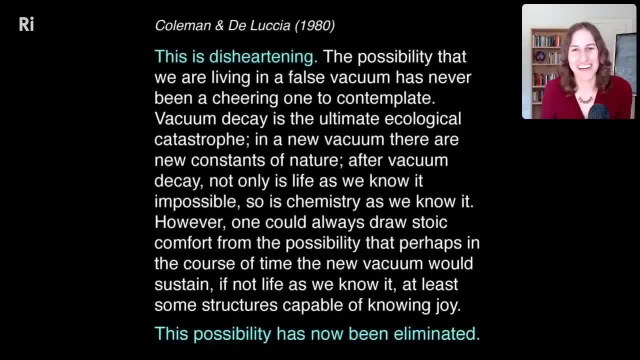 So it sounds bad, right? I've just told you that there's this random event that could happen anywhere, destroy the whole universe and nothing capable of knowing joy could survive it. But there are a couple of reasons why you shouldn't worry about this. I did promise. 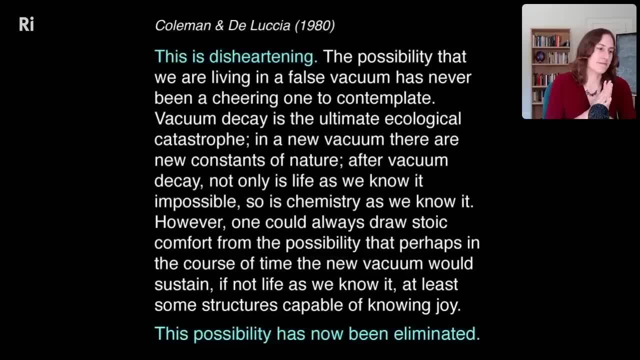 I would tell you not to worry about this. One reason is obviously there's nothing you can do about it. You couldn't see it coming, You couldn't stop it. Why worry about something like that when you could worry about things that actually are under your power to effect? 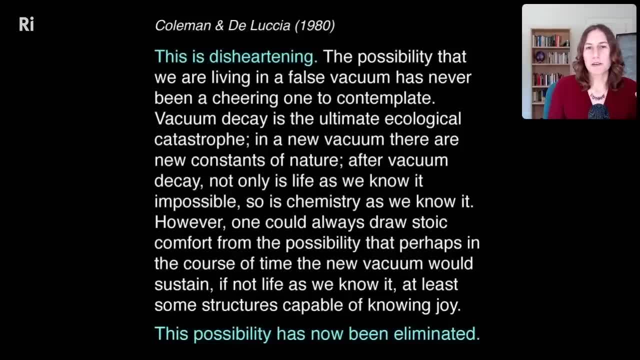 Even aside from that, the, as far as we know, the probabilities for this happening anytime soon are just astronomically low. So we can calculate them. We can calculate the expected time to a tunneling event. We can't calculate exactly when's it's going. 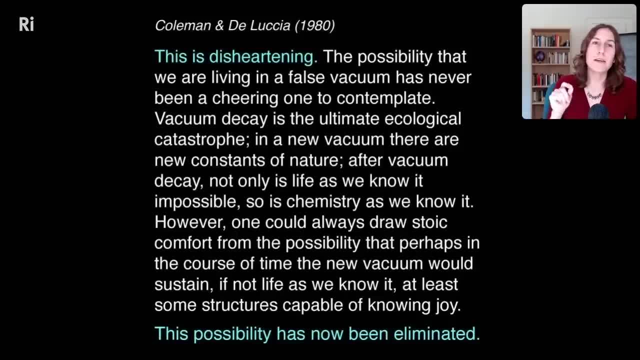 to happen. We can calculate the expected time, and when we do that for vacuum decay we get a number of 10 to the 100 or 50 years. That's a very long time from now, And the chance of it happening any time soon would be much less severe than a 10 to the 50 year old development. This is true一个. 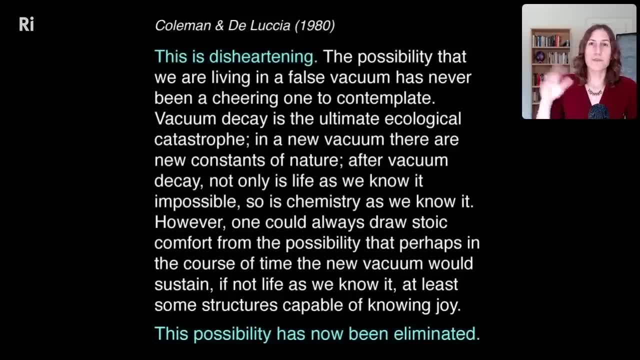 soon is is so astronomically low. it's like everybody on earth winning the lottery ticket at exactly the same time while being struck by lightning or something like that- like it's a very, very, very, very tiny probability, um and uh, and anything that has ever happened to anybody in. 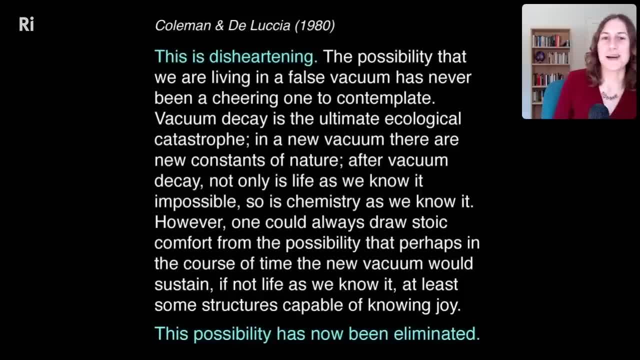 the history of the planet is more likely to happen to you than vacuum decay is? um, just based on what we know about it, uh, from from our calculations, but um, the other reason that that you really shouldn't worry about vacuum decay is that the vacuum, the idea that vacuum decay is even possible, 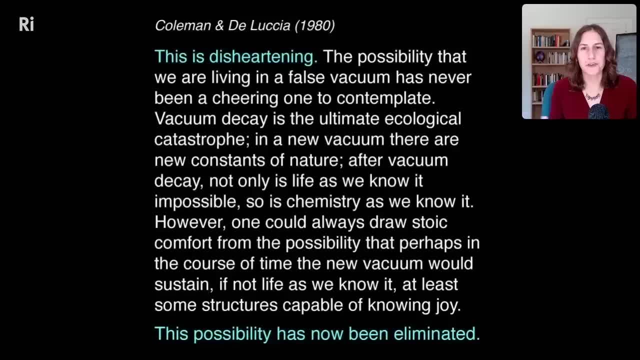 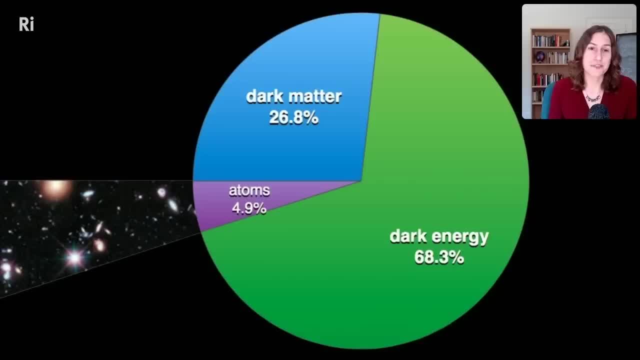 is based on the idea that the standard model of particle physics is really totally correct, that that we know what we're doing by calculating things in the standard model of particle physics. and if you look at what the universe is made of, what we know about the cosmos, we know that. 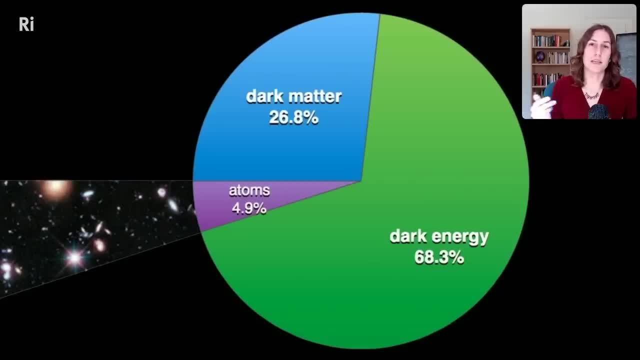 most of the universe is dark energy. which is this mysterious stuff that we don't understand? we don't know exactly how it works? um then, after that, the rest, most of the rest of the universe is made of dark matter, which is a kind of invisible matter, that. 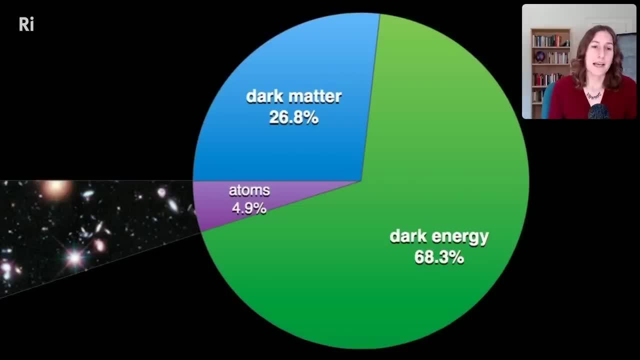 we also don't understand. we're pretty sure it's out there, but we don't know what it's made of. and um, then there's just this little sort of five percent slice of the universe that contains everything we've ever measured in a laboratory, everything we've ever seen or touched. 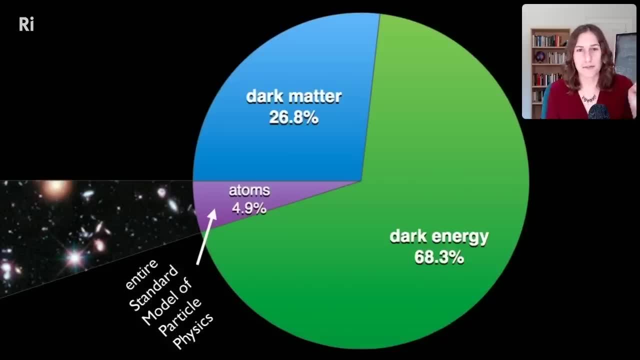 and the entire standard model of particle physics lives in that little standard, that little five percent slice. so everything we're basing this idea of the end of the universe on comes from this, this very insignificant part of of what the universe is made of, and so it's very possible, and maybe i would say even likely, that when we understand what dark matter, 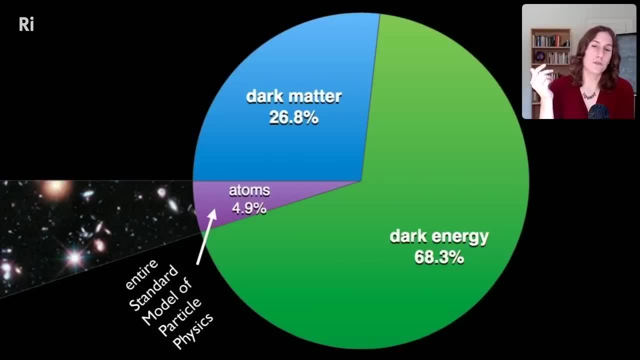 and dark energy are. that will change our our view of the future of the cosmos so completely that the idea that vacuum decay can happen in the way that we're talking about it will not will not be on the table. we'll figure something out that'll change what we expect for vacuum decay, or and for all. 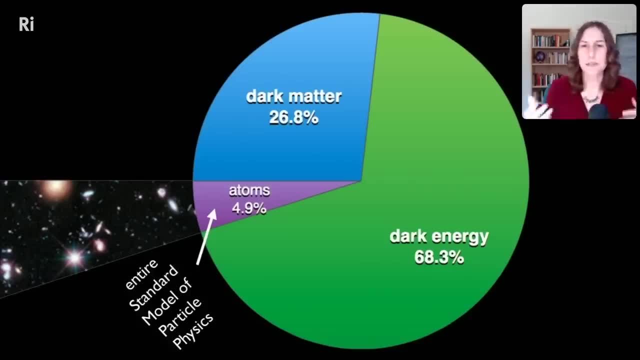 these other scenarios as well. um, i didn't get into uh other possibilities, but i think that's a good question. um, i would say i think that's a good start. um, but, as i mentioned, i wanted to give a quick overview of the universe because there's uh a lot of different possibilities for the universe. 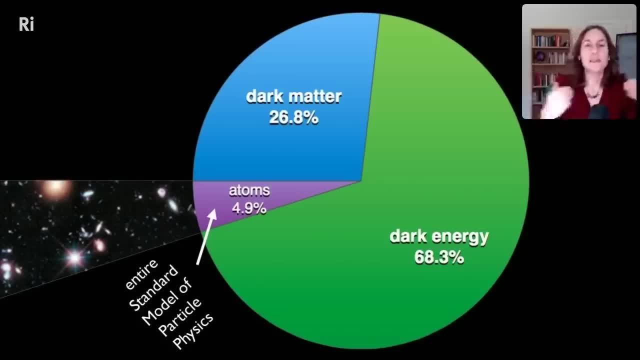 there's the. there's things like bouncing cosmologies, where you could have a universe that cycles from a crunch to a big bang, and so on, over and over again. um, and that's those ideas are based on rearrangements of our understanding of the early universe and the structure of the. 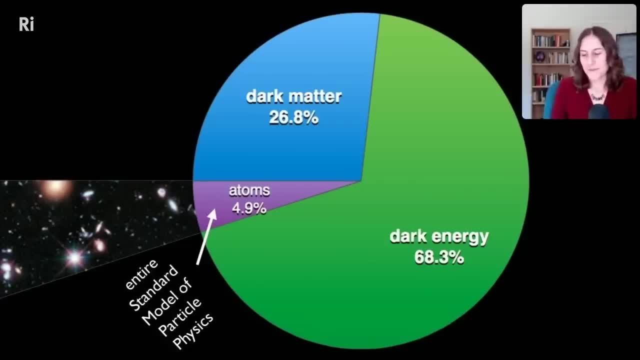 universe and sometimes you can have more dimensions of space and that can give you a different evolution of the cosmos. so there's so much that we don't understand about the universe to be specifically scared of any particular ending. So the point is that when we do this, 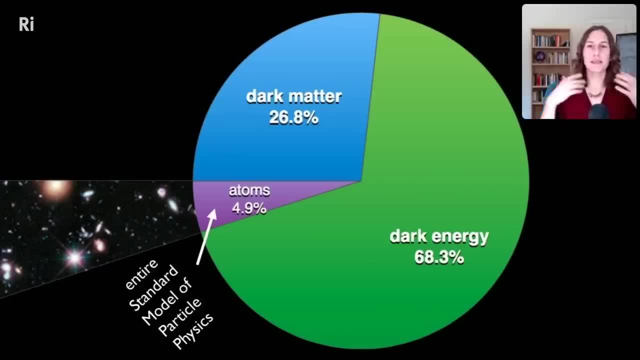 exercise when we think about the future of the cosmos, when we extend our curiosity and our extrapolation into the future, when we take what we know about the cosmos and we can and figure out what's coming next. it can be an amazing exercise for examining the assumptions. 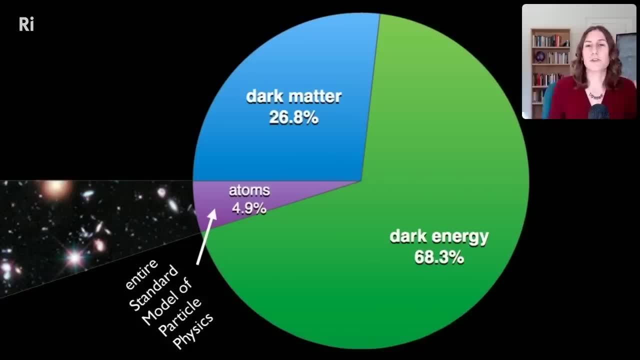 that we build into our physics models, examining the structure of physics as we know it, and it can be a way to think about also how we fit into this bigger picture as humans. you know as little, tiny specks of dust in that five percent slice of the universe. Where do we fit into this bigger picture? 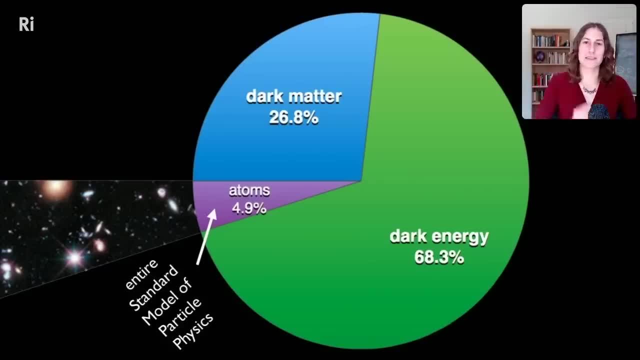 What does it mean for us as a species if we're this tiny, insignificant speck and then the whole universe is going to end? How do we conceptualize our existence? So I think it's definitely an important thing to think about. I think it's a useful exercise to go through and I hope that by thinking about these big questions, 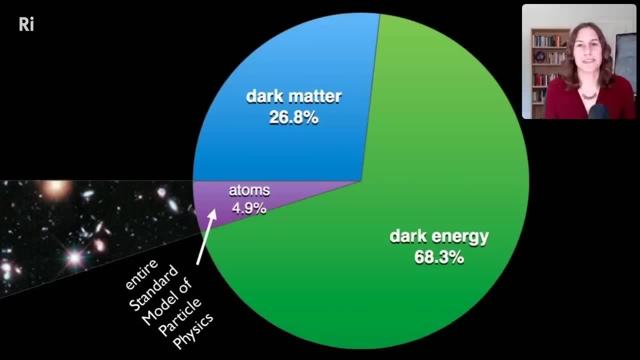 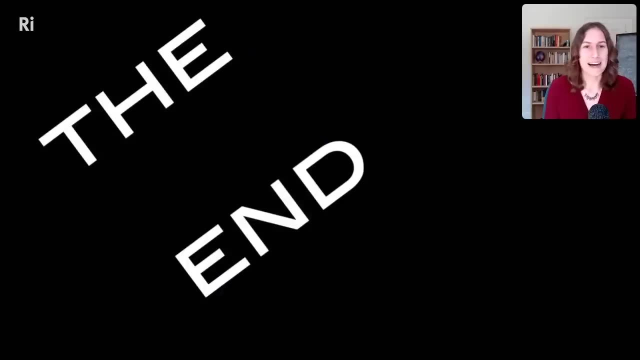 it helps you to think a little bit differently about how we all fit into the universe and how we can kind of make the most of what we have in this cosmos while it's still here. So I will end there and thank you very much for being here, and I think I will be answering some questions. Thank you very much.